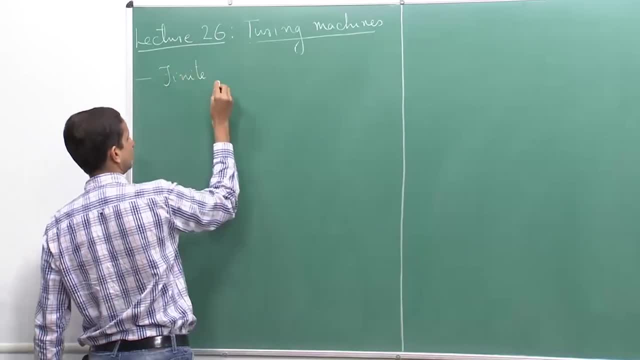 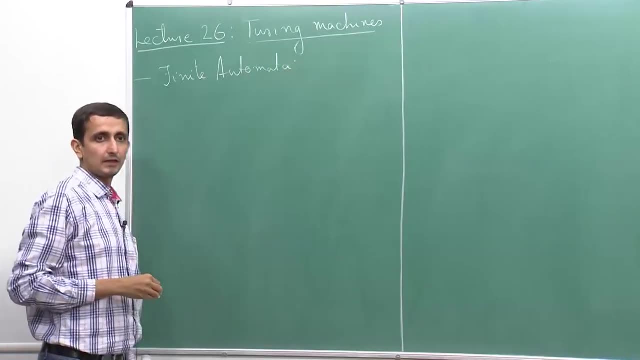 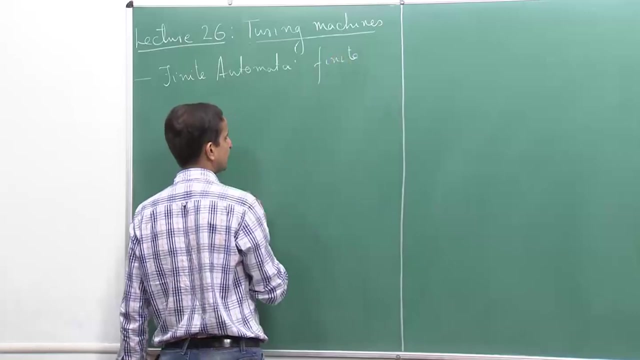 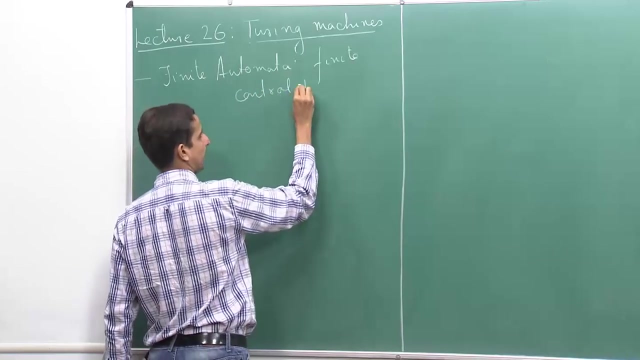 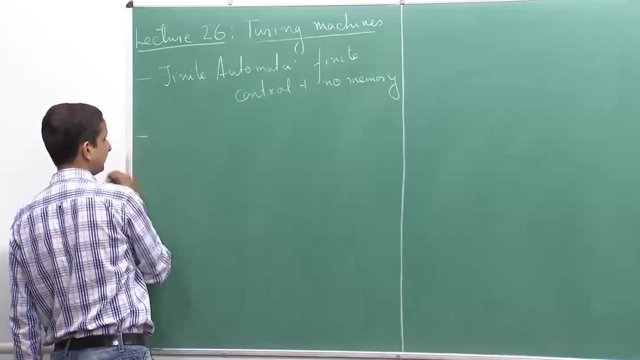 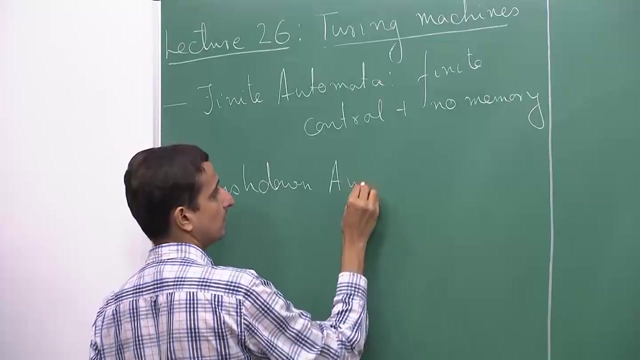 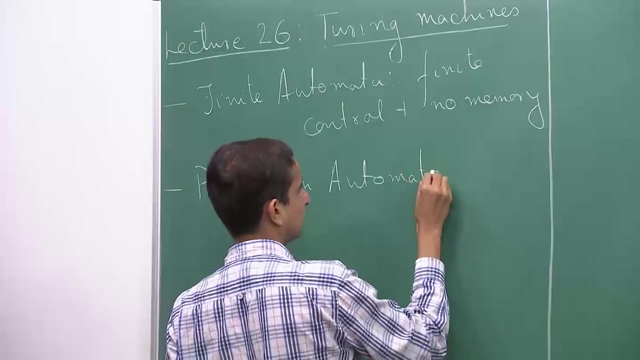 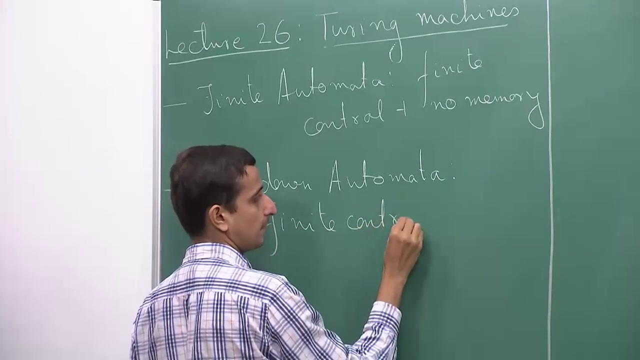 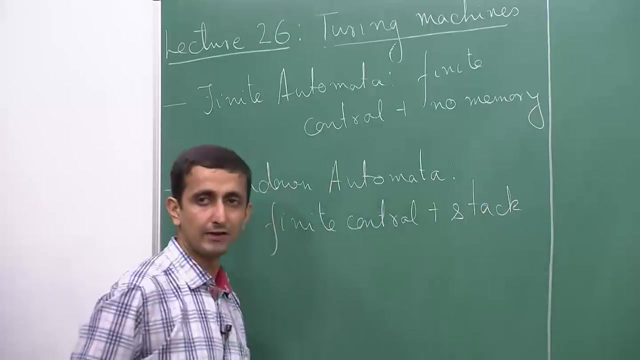 automata. In finite automata we had a finite control and no memory. Then we introduced push down automata. So in push down automata we had a finite control plus memory in the form of a stack, So by finite control essentially. 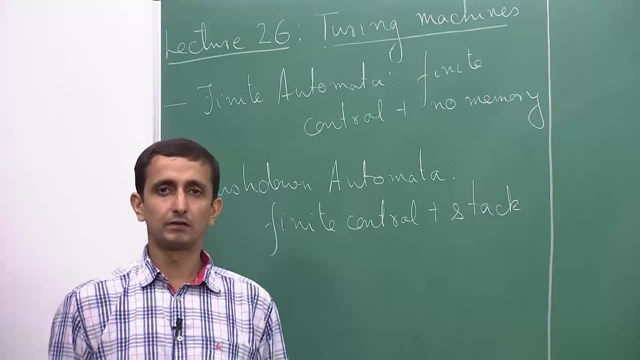 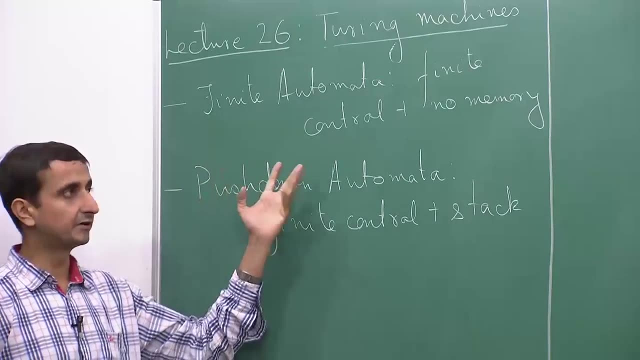 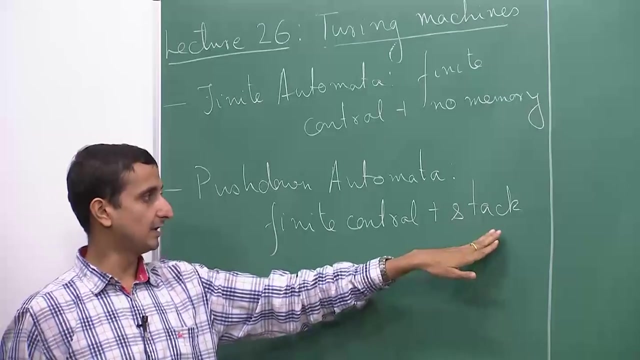 we mean that the set of states is finite in nature. So in finite automata, both deterministic and non-deterministic, we do not have any memory in that model. But in the case of push down automata we have an unbounded stack as our memory. So there, 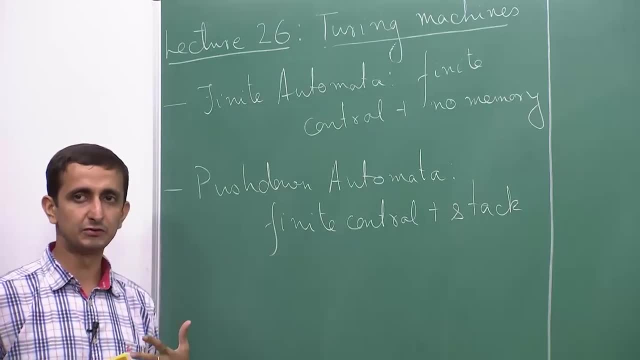 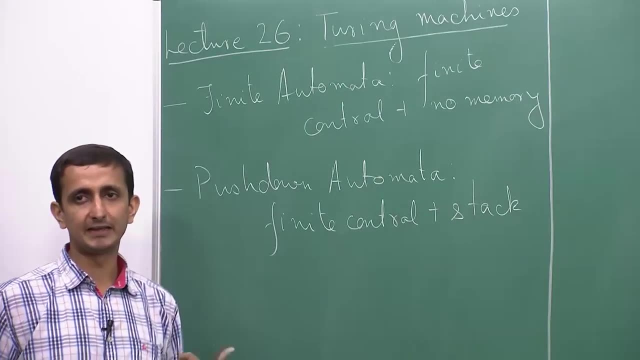 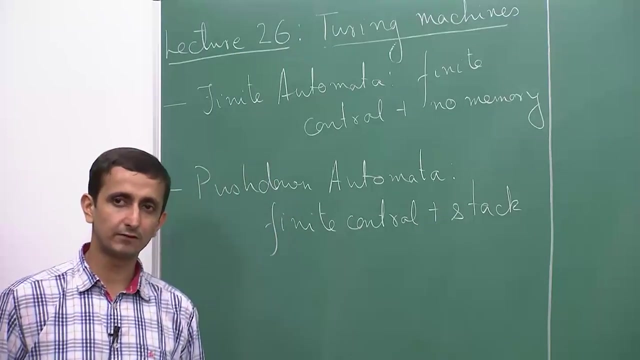 is no bound on the length of the stack that can be used. the only restriction is that it is a stack. therefore, we can only access the topmost element at any given point of time. So now the question is that: can we, how can we extend this? So, instead of a stack, 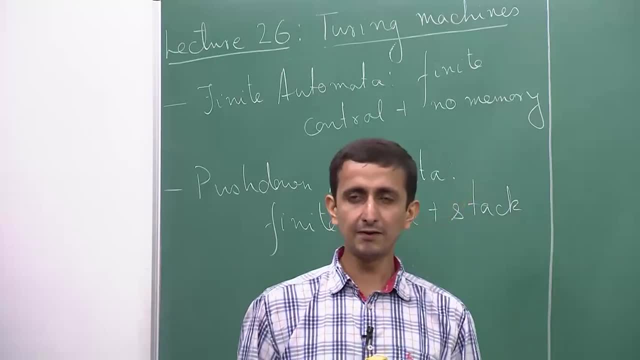 what if we consider other data structure? So a Turing machine is essentially a set of elements. So a Turing machine is essentially a set of elements. To do this it has to be connected to a certain number of units. So a Turing machine is essentially a set of elements. So 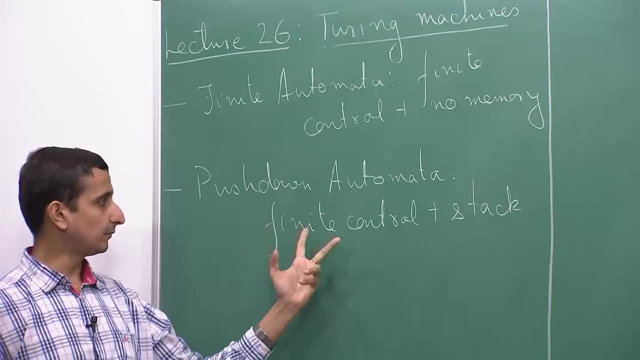 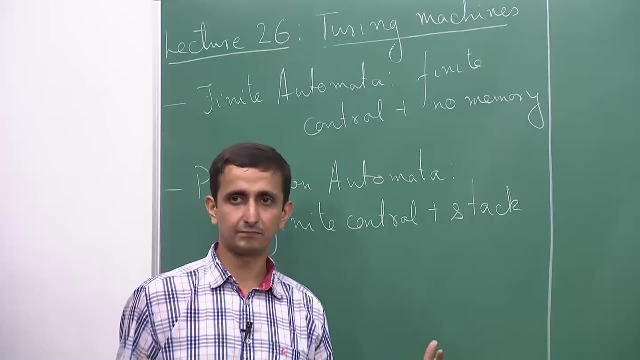 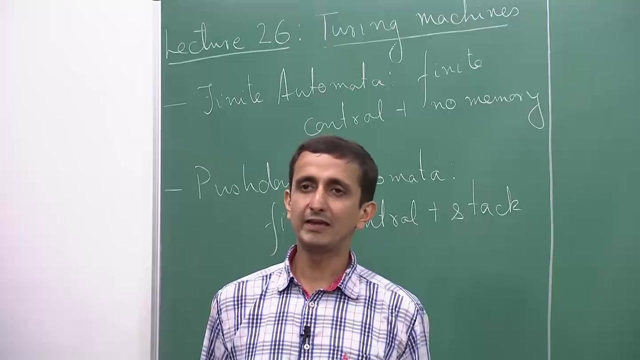 An automata where we have finite control plus memory, in the form of a tape instead of a stack. So what is a tape? A tape is again an infinite data structure, but in the case of a tape, we can access any cell at any given point of time. 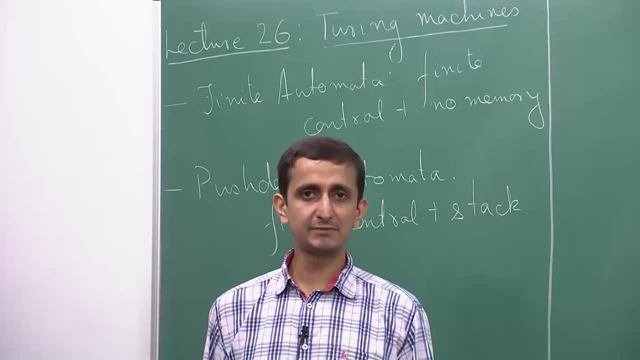 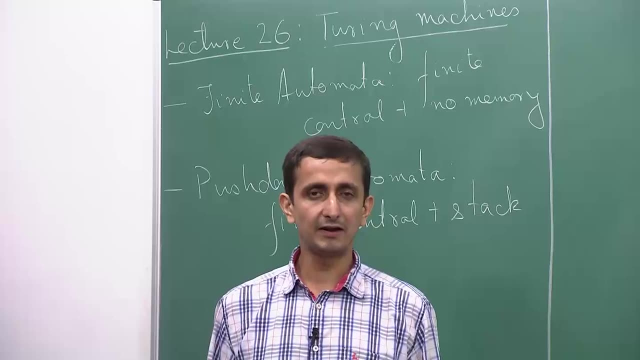 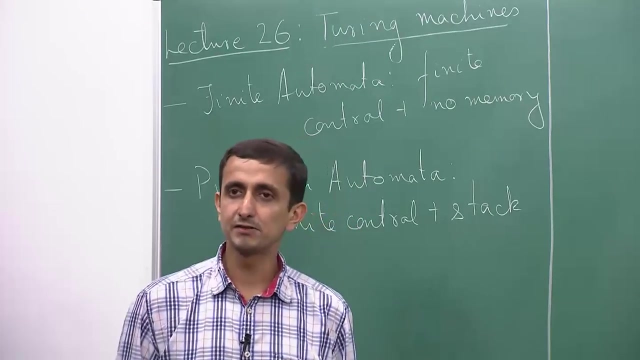 So a tape has a tape head which is pointing to some cell of that tape and we can move the tape head left or right, whichever way we want, and access whichever cell we want to. We do not have to erase contents of the tape to access a certain cell, as we had to do in. 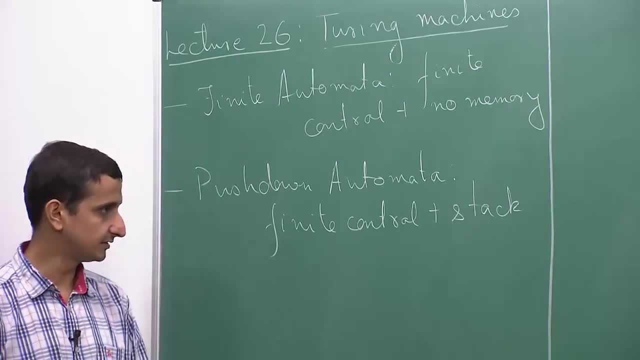 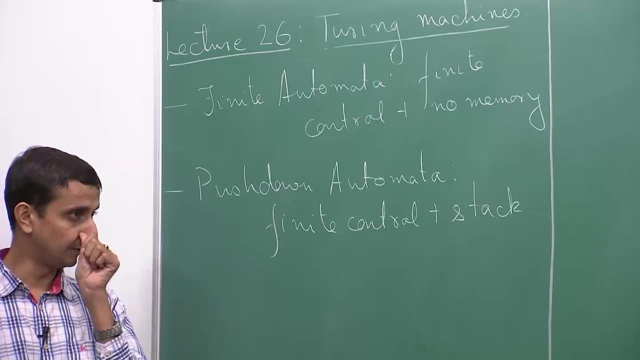 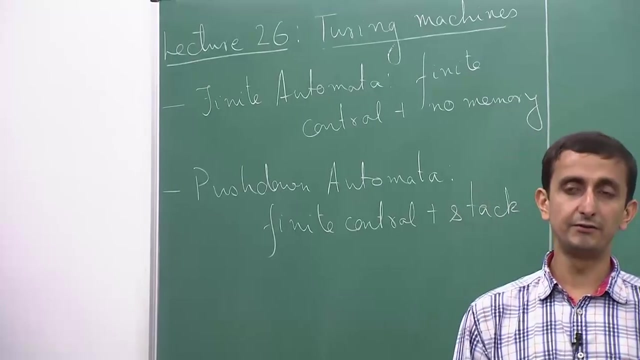 the case of a stack. So that is essentially what a Turing machine is. We will see more formally what is the definition. how do we define a Turing machine? but before that let me give a brief historical model Motivation as to how Turing machines were invented or how they were discovered. 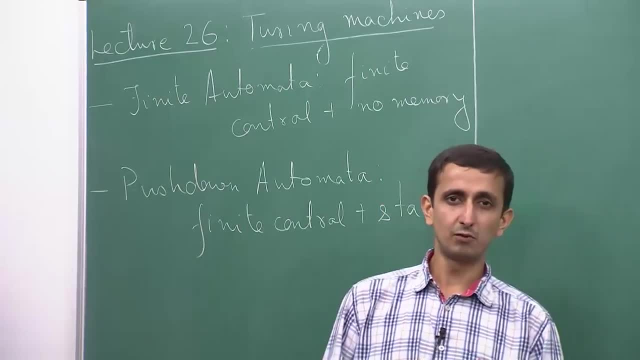 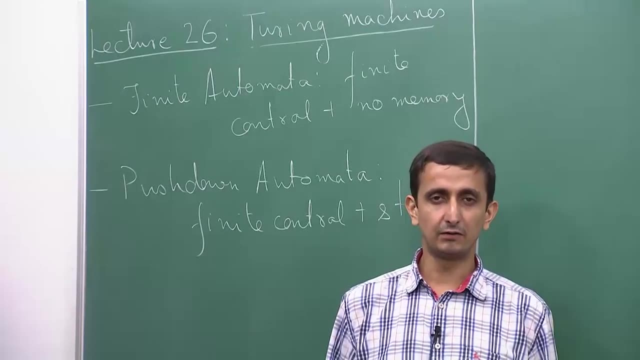 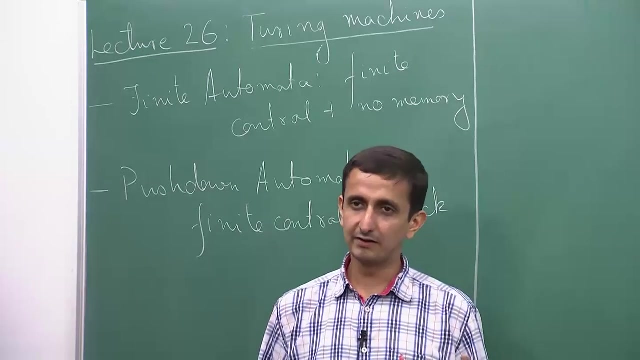 So a Turing machine. somewhat contrary to what the name suggests, it is not a mechanical machine. it is not a machine in the sense that we colloquially use it. It is a mathematical object. it is basically an automaton. it is a mathematical object. 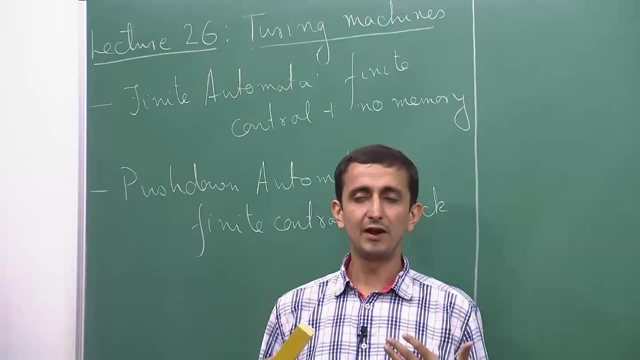 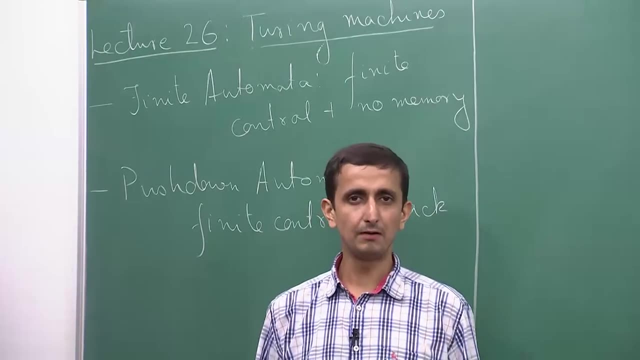 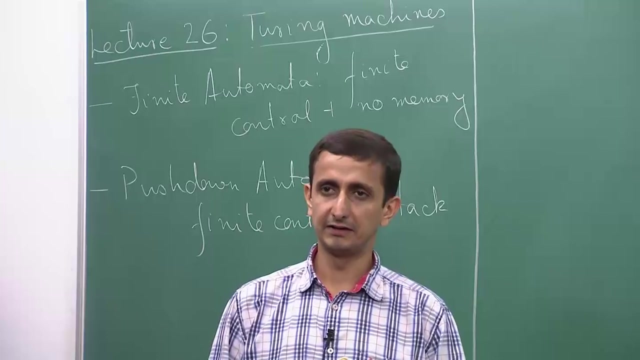 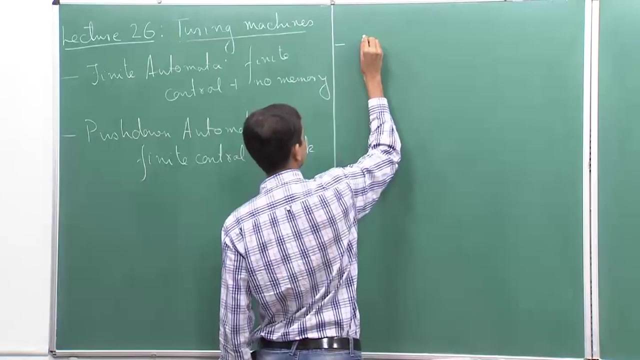 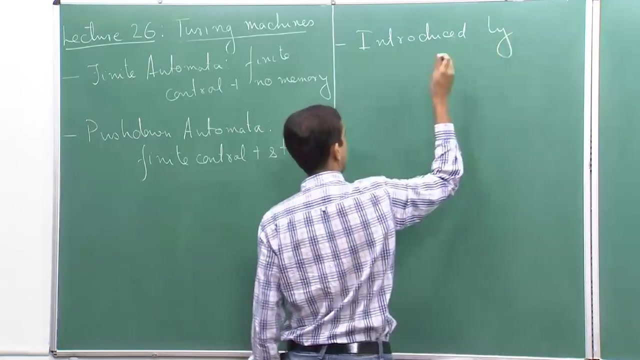 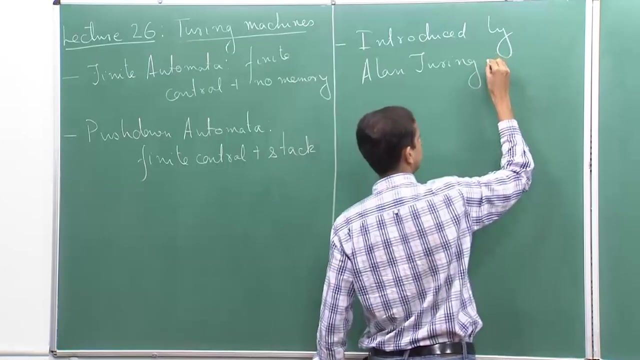 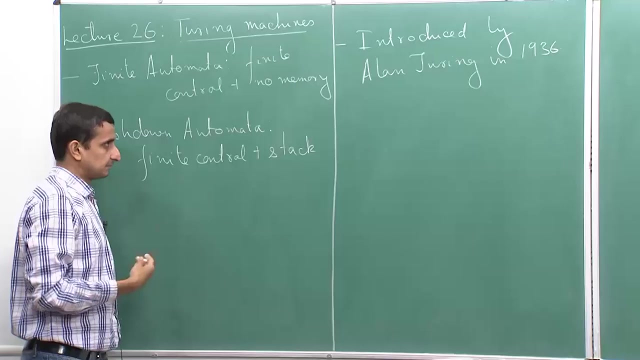 which is modeled to simulate computation. So any computation can be modeled in a Turing machine in a similar way that it had been done in the case of finite automaton and push down automaton. So Turing machine was introduced by Alan Turing in 1936. So the historically it is very interesting how Turing machines 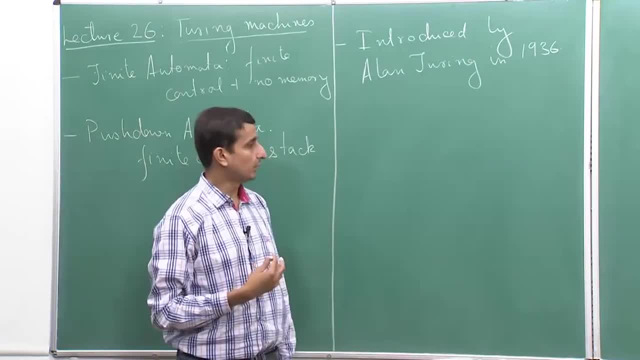 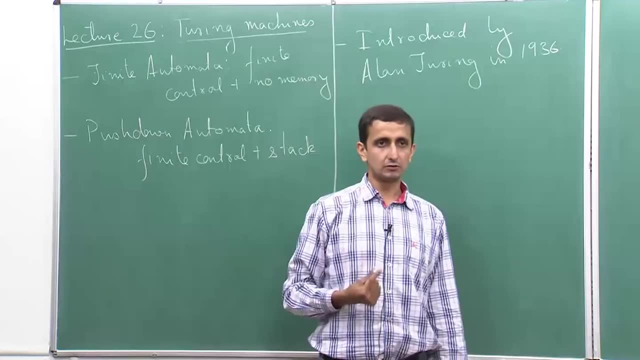 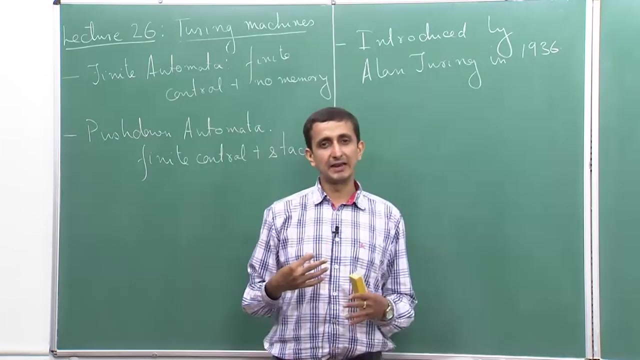 were actually discovered. So what Alan Turing was trying to do is: Alan Turing was trying to understand the limits of computation. So are there any computational problem which cannot be computed in the sense of the word? So they were. so in 1936 we did not have 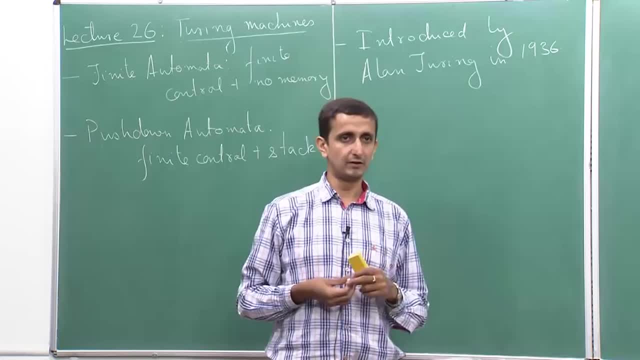 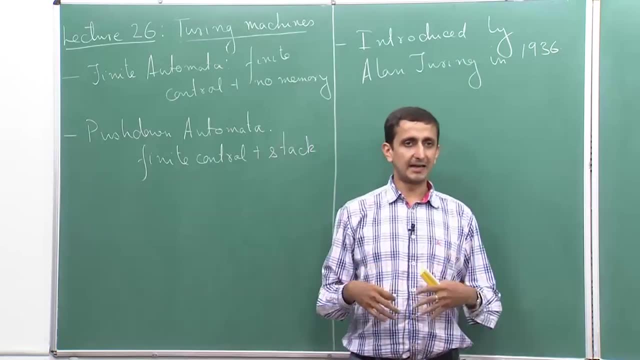 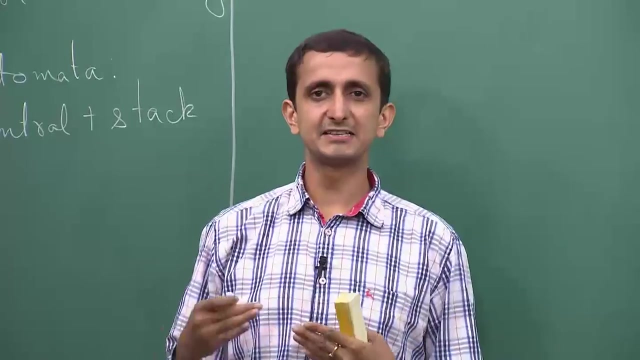 computers, computers that we see today. So, but the definition of computation was sort of clear. I mean any process that can be used to obtain an answer from a given input using a step by step process. For example, if I want to multiply two numbers, I can always. 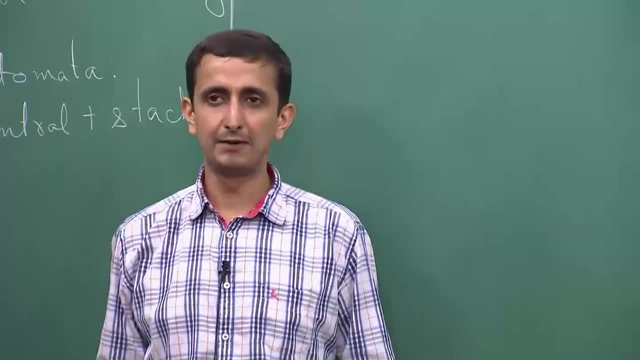 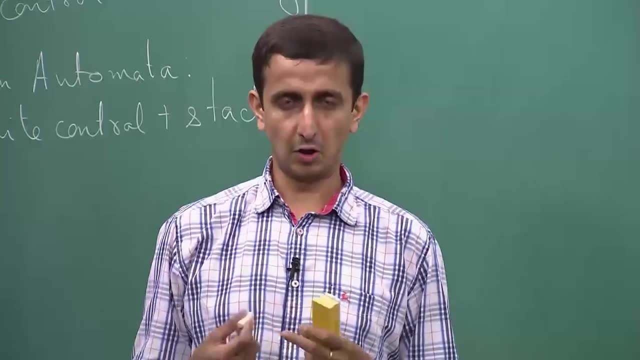 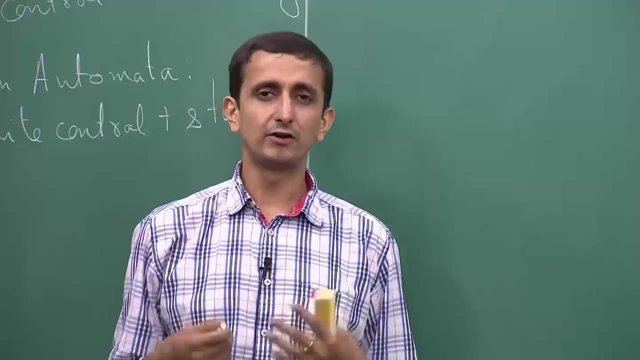 do that on pen and paper. I can always devise an algorithm that would tell me how to go ahead multiplying two numbers in a step by step manner to obtain the product of the two numbers. Similarly, for other problems also, there are methods that you can apply in order. 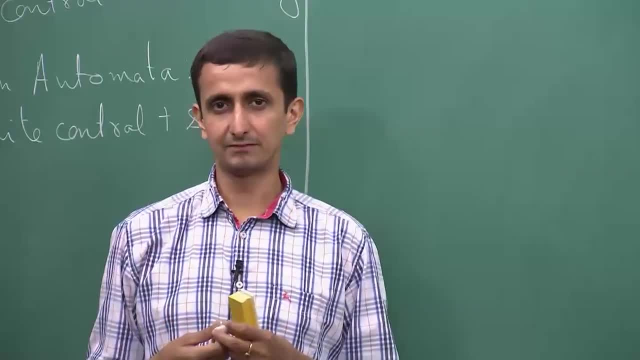 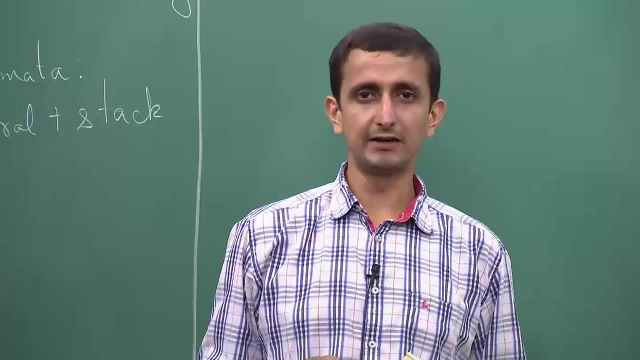 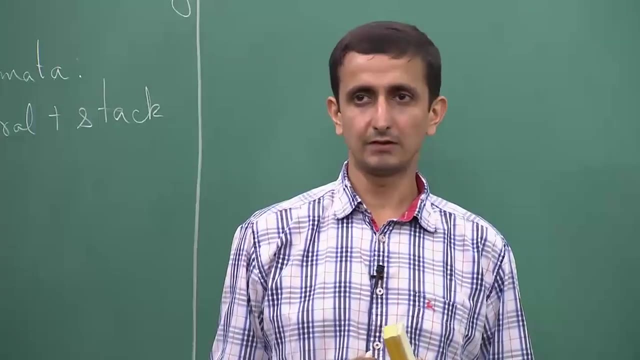 to get the solution from the input in a step by step manner. So the question that Alan Turing or even mathematicians before Alan Turing were interested in is that: is there any problem? is there any computational problem where you cannot actually obtain a solution by going in a step by step manner? And to actually prove this, 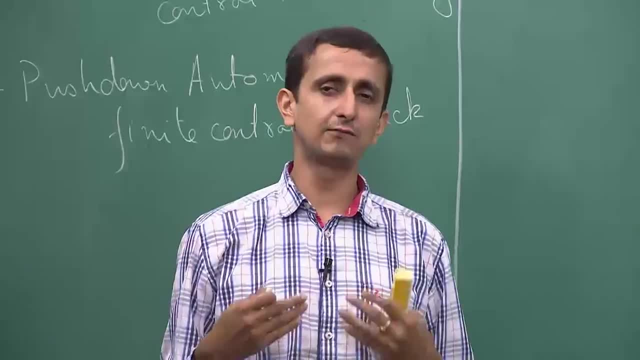 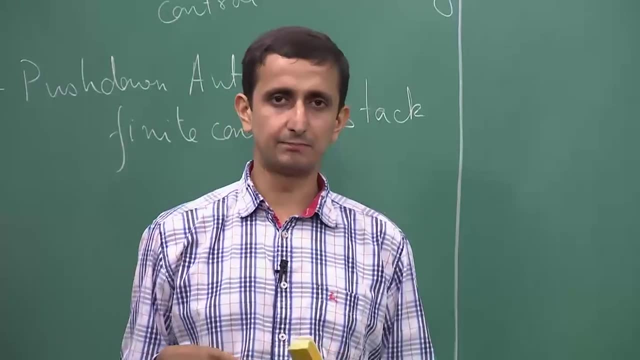 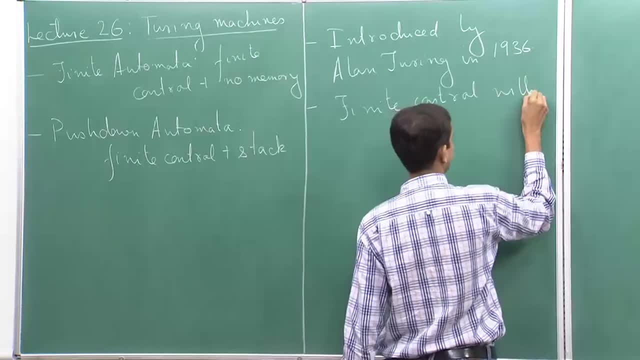 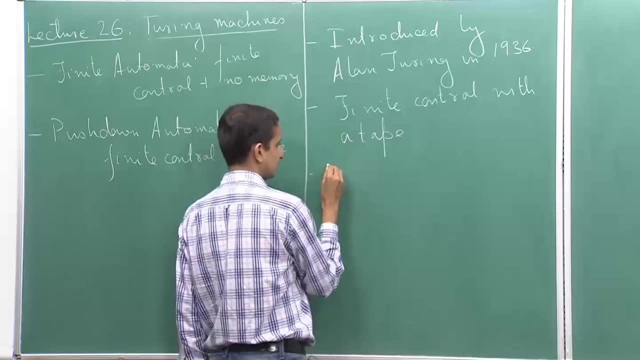 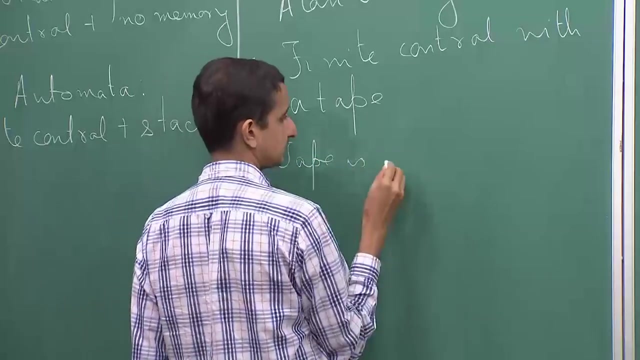 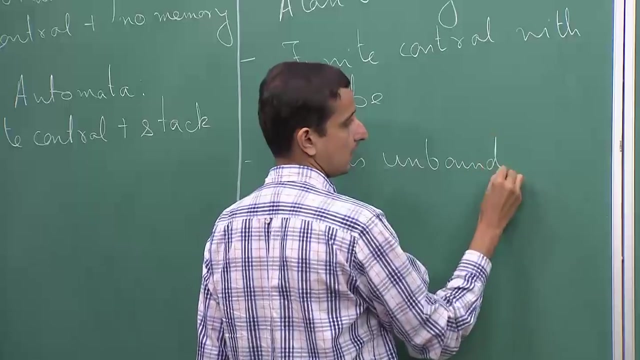 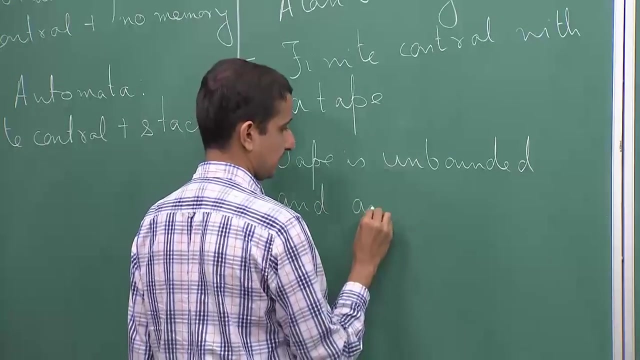 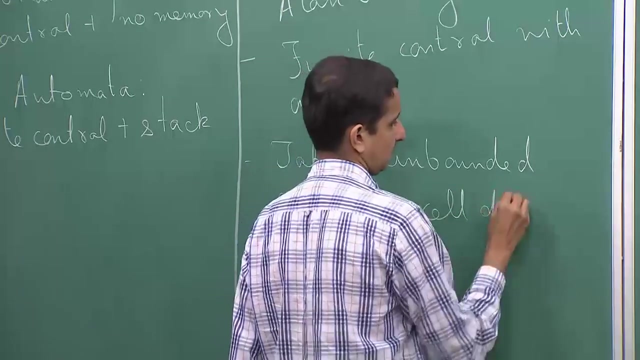 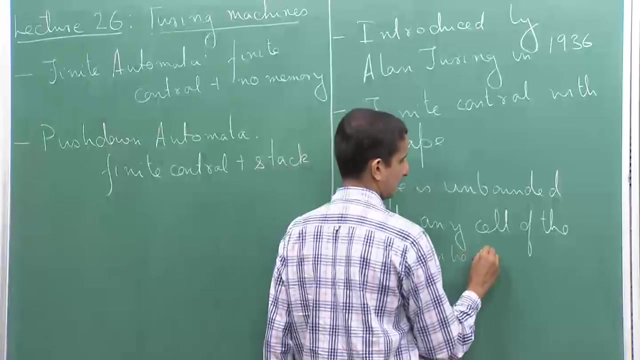 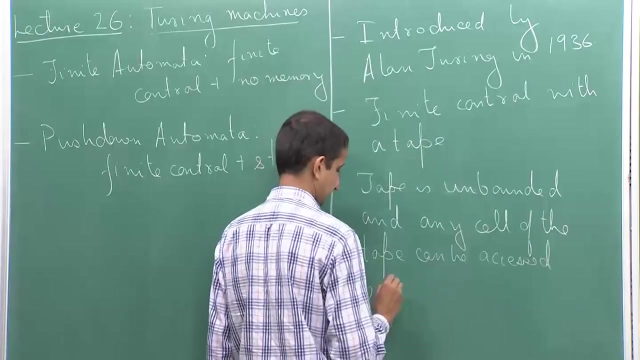 prove this, it is essential to give a mathematical modeling of what computation is. And to actually prove this, it is essential to give a mathematical modeling of what computation is And to actually So. the tape is unbounded and any cell of the tape can be accessed. 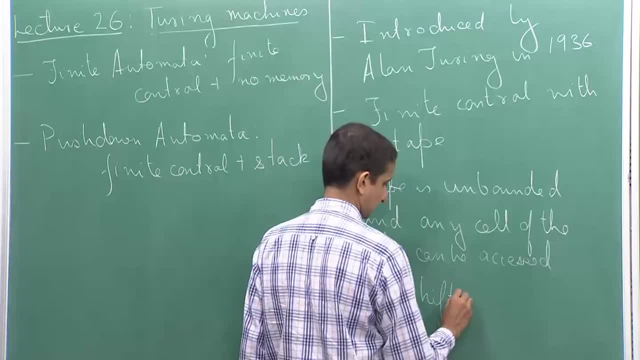 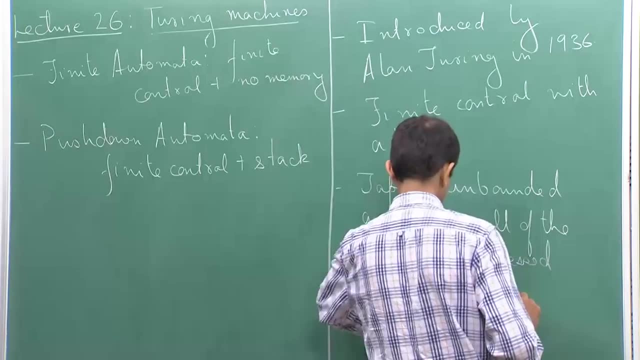 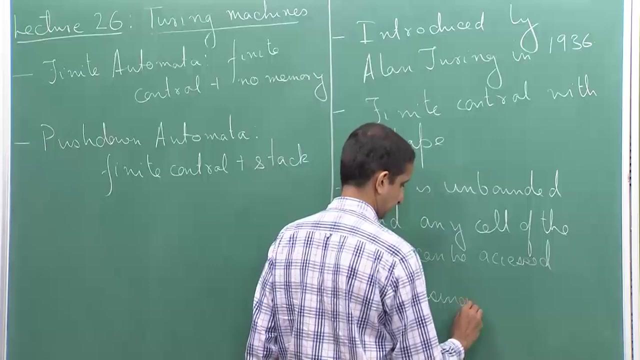 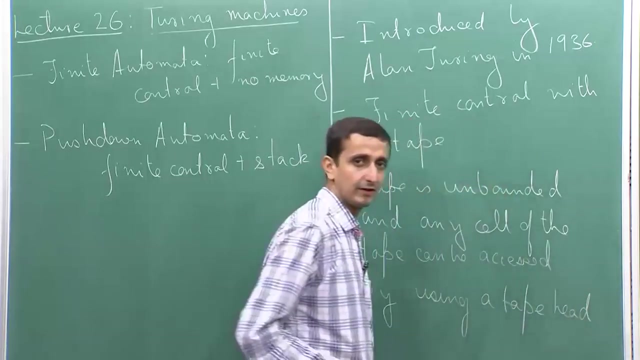 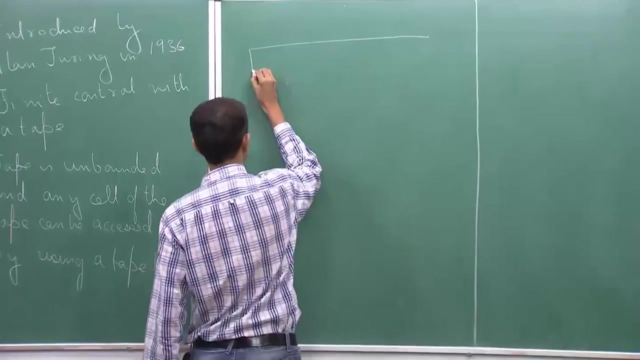 by the tape. So the tape is unbounded, So the tape is unbounded By using a tape head. So let us look at a picture. So, essentially, a tape is unbounded in nature, So it is more precisely, it is semi unbounded. 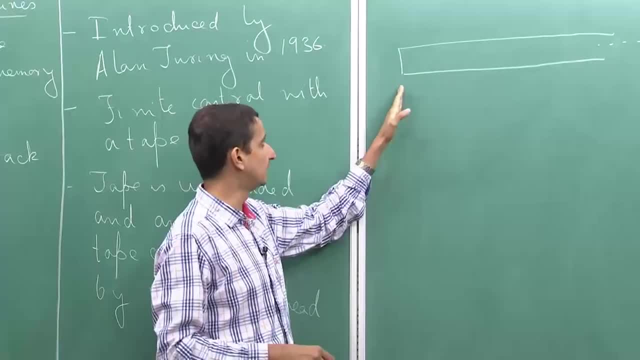 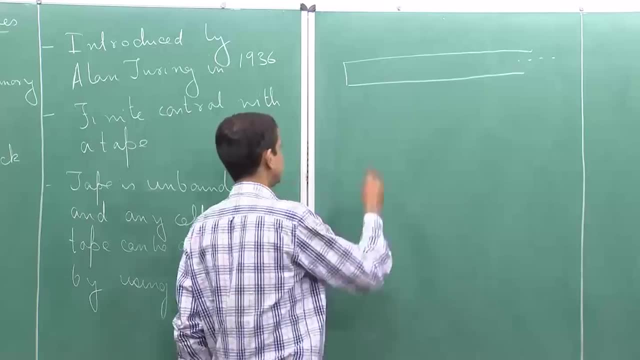 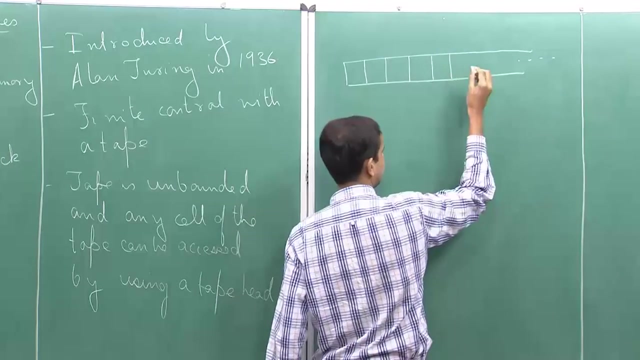 So in the left side there is a bound, So you cannot move to the left of the. this boundary on the left, but on the right side it is unbounded. So this is how you can picture. And it has cells. so every cell has is capable of containing one symbol and there is a tape. 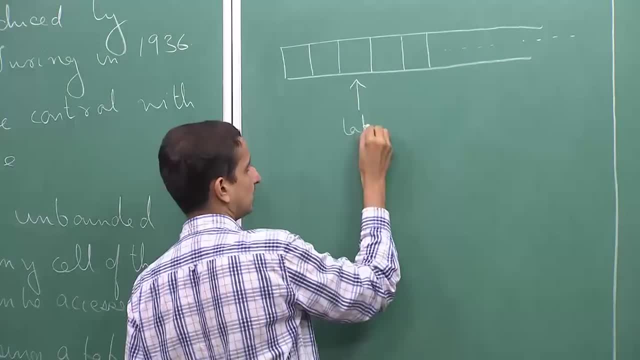 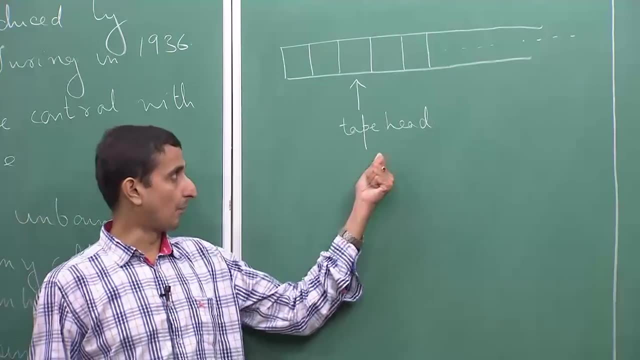 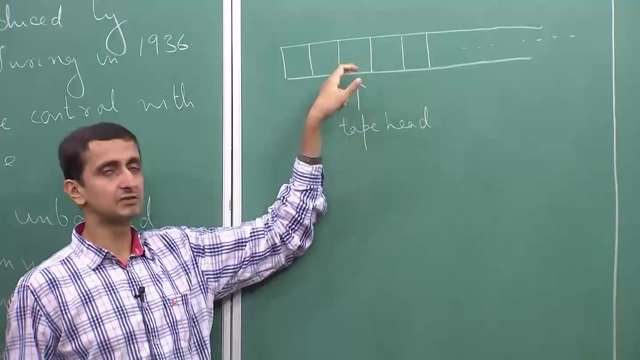 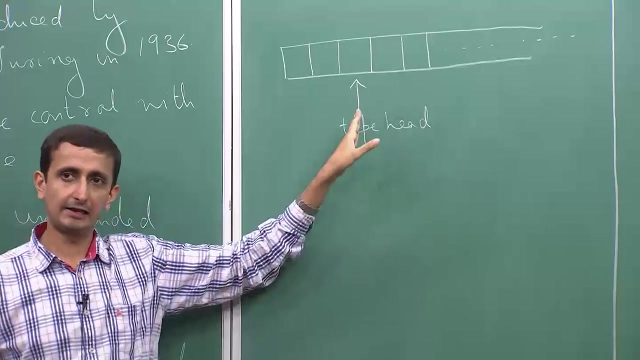 head. Okay, So this is The tape head which is capable of pointing to any cell of the tape, And whichever cell the tape head points to, you can read the contents of that cell only. Okay, Now suppose, if you want to read the content of this cell, then in two moves. first the 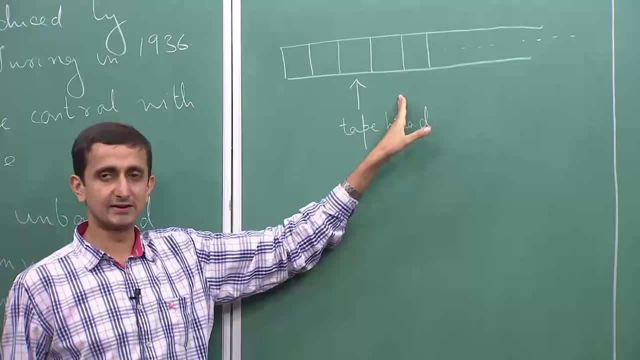 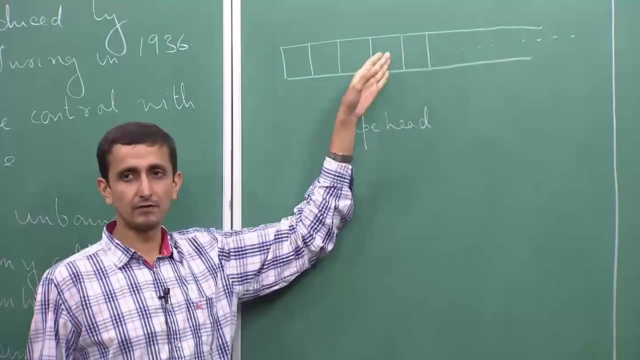 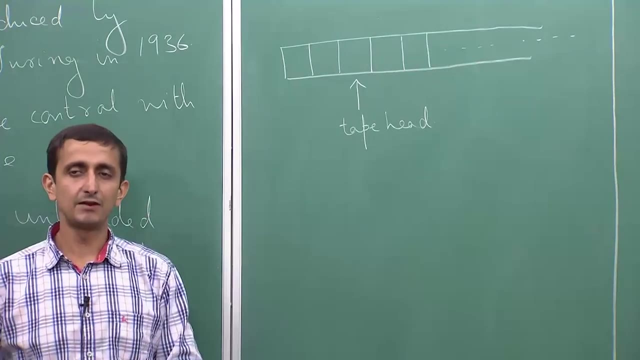 tape head has to move from this current cell to the one to its right, Okay, And then again, in the next move, it has to move one more step to the right, and then you can read this: Okay, So in every step, basically, you can move the tape head either to the left or to the right. 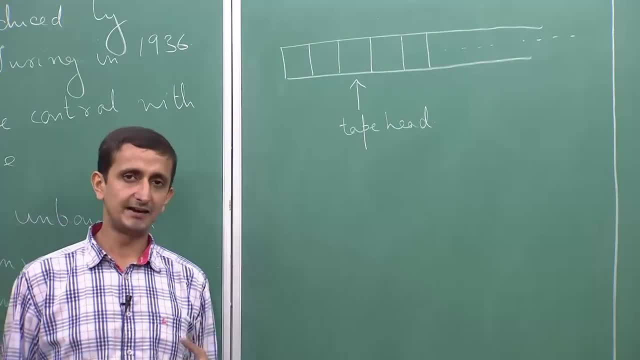 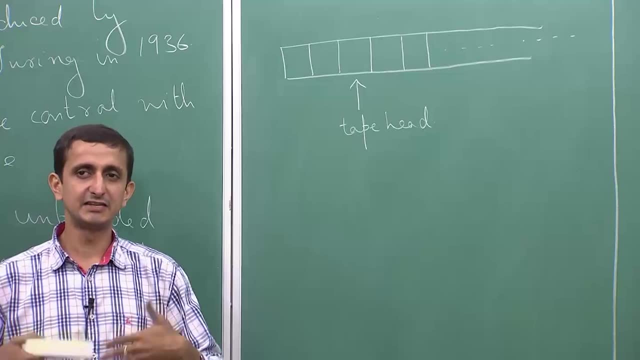 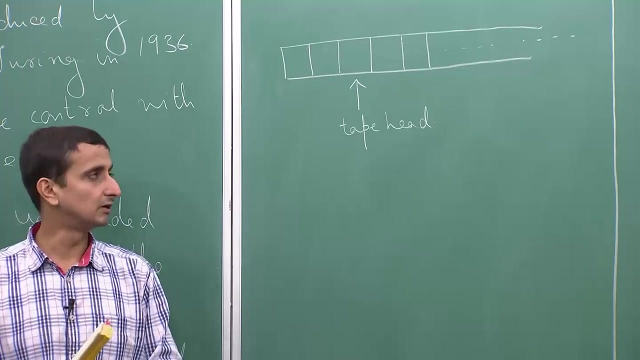 And you can read the contents of the cell to which the head is currently pointing to, And you can also modify the content You can modify to. you can basically change whatever symbol is contained in that tape cell to anything that you want. So this is how a Turing machine works. 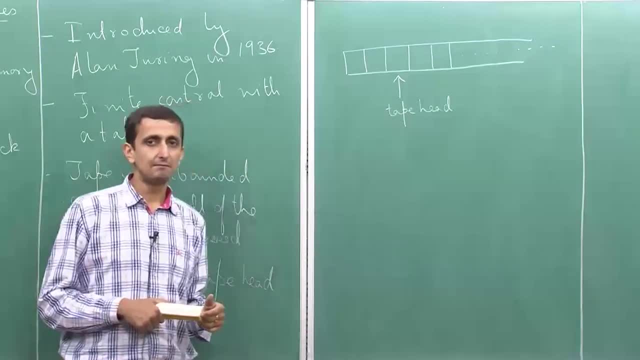 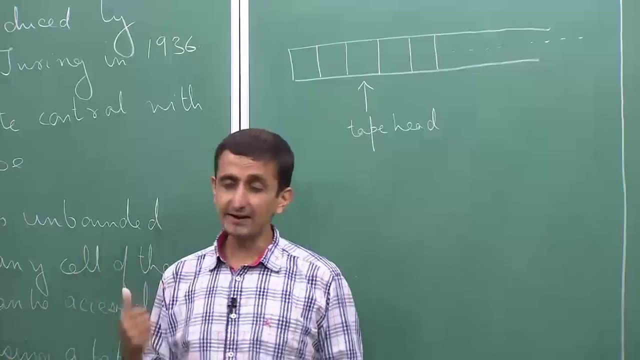 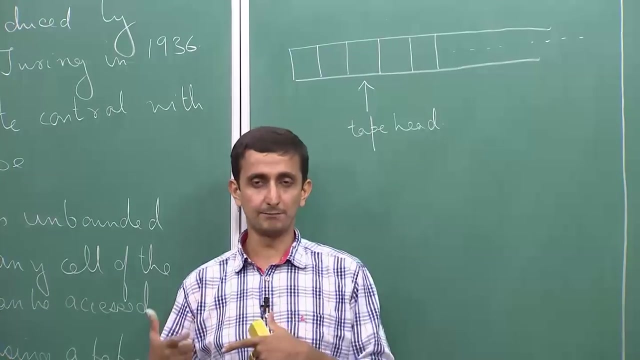 Okay, So essentially the tape corresponds to the memory of the Turing machine. Okay, So, if you want to think of this as a computer, so the finite control is essentially the CPU of the Turing machine of the computer. Okay, So the finite control is able to decide where your tape head should be. 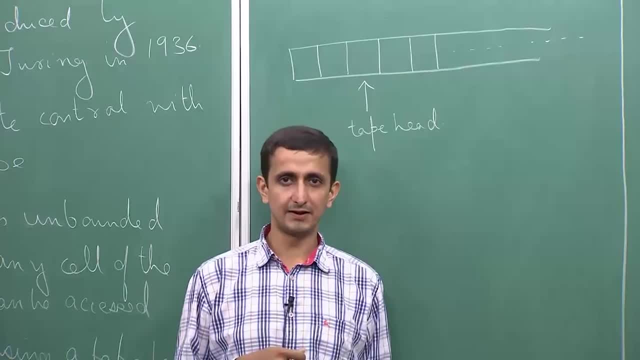 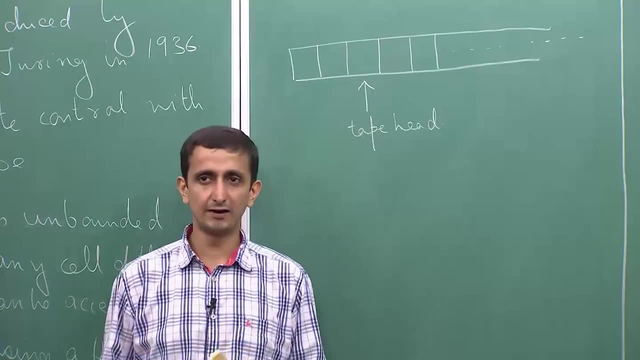 Where your tape head should move, to what contents it should be replaced by. So suppose, if you are running an algorithm, your finite control is essentially the steps of the algorithm, what essentially you need to do at every step, And the tape is essentially the memory that your algorithm uses. 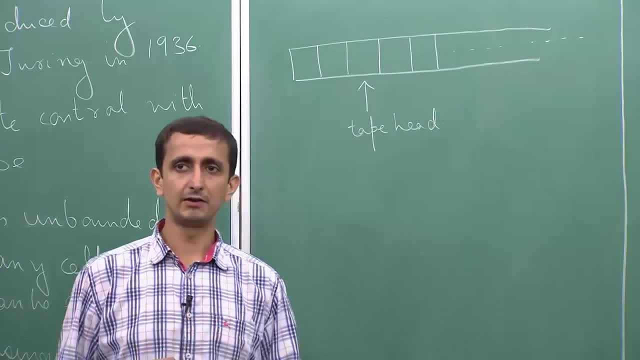 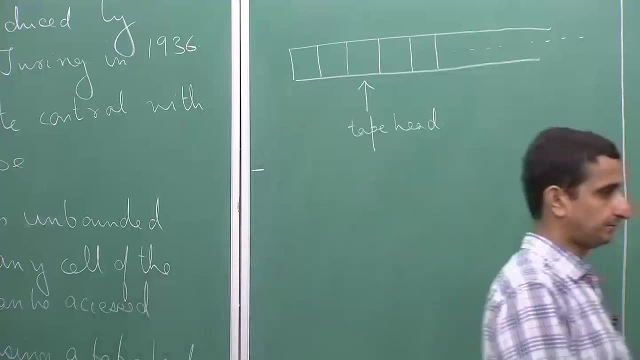 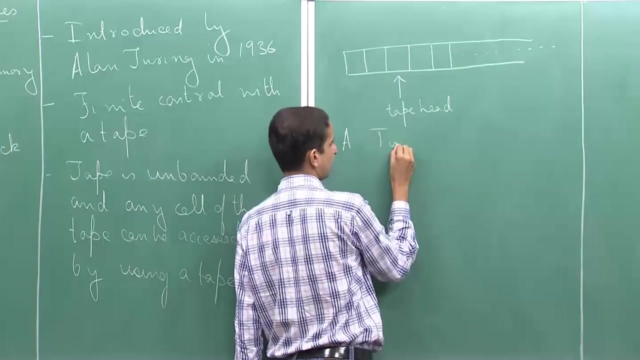 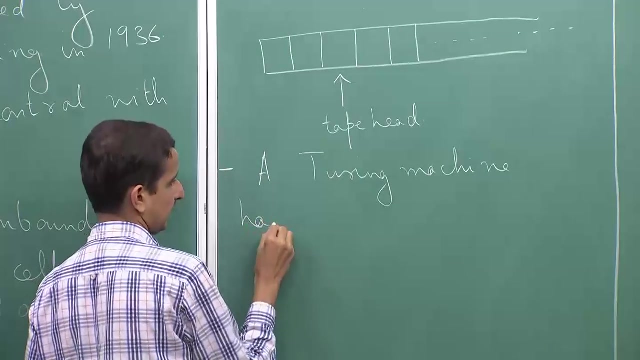 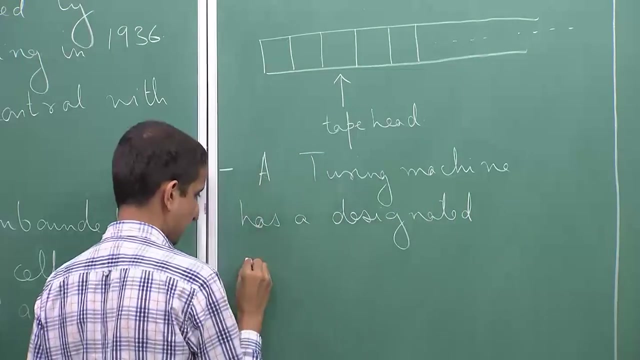 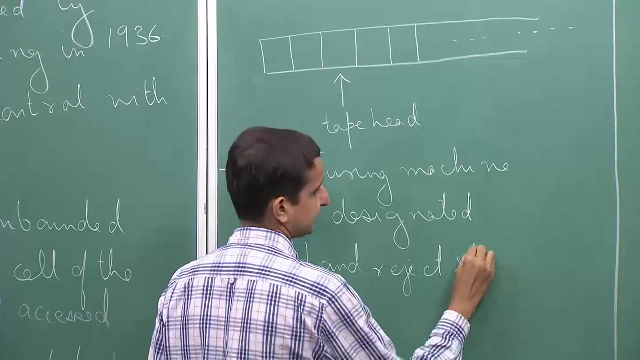 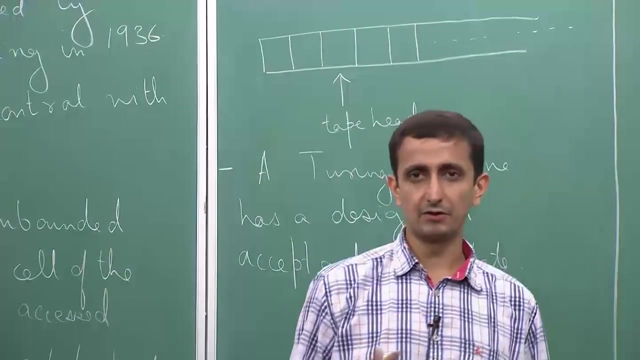 Okay So, whatever content that you want to save in order to compute something, Okay So, So a Turing machine has a designated accept and reject state. Okay So, this is again something that is different from a push down automaton or finite automaton. 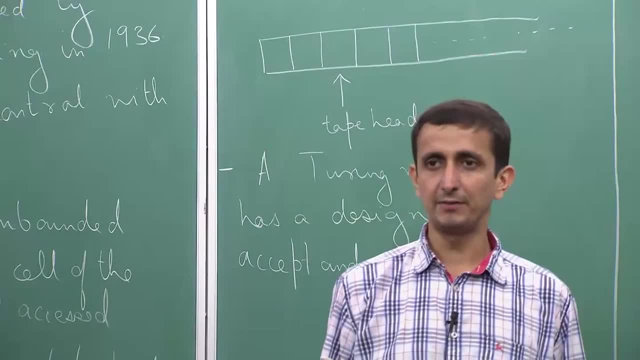 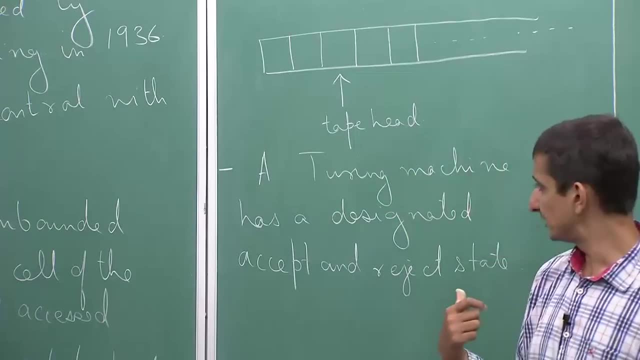 So in the case of a finite automaton, or let us say push down automaton, there was an input tape where the input was written. But in the case of a Turing machine we will assume that the input itself is written on the tape of the Turing machine. 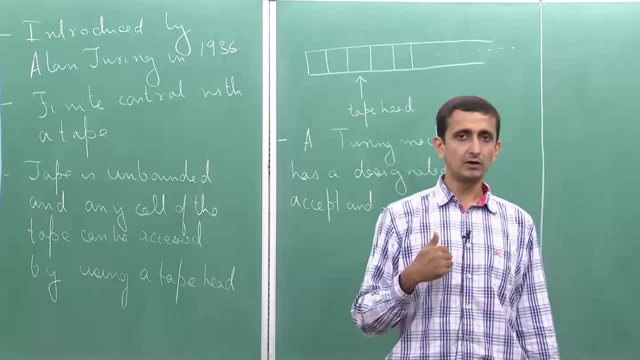 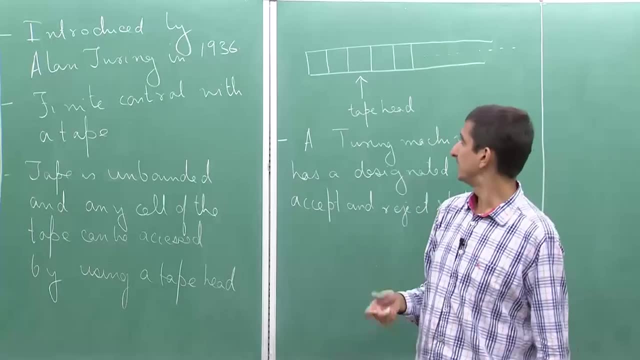 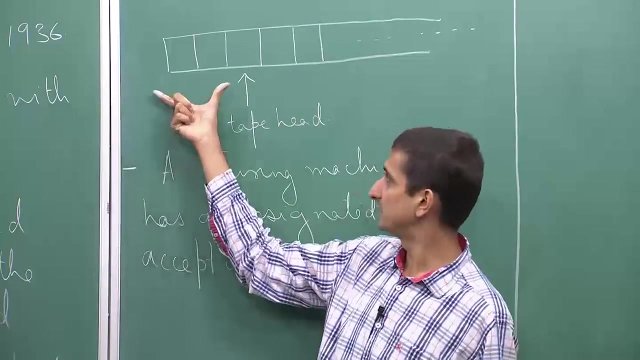 So that we will assume that a Turing machine has only one tape which is used as workspace as well as to store The input. Okay, And we will assume that the input is written to the left left hand side of the tape. Okay, 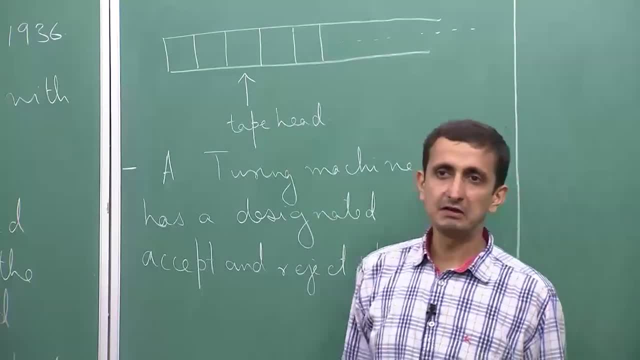 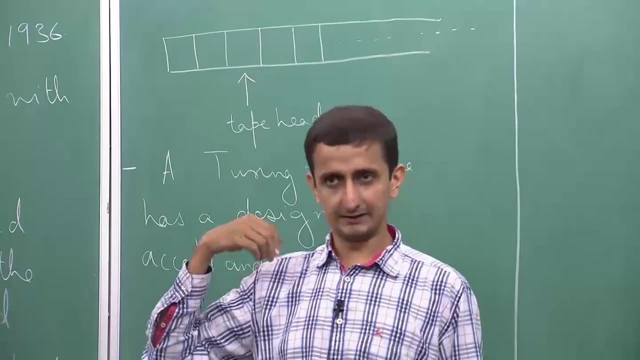 So whatever input is, it is written on the left hand side And then you can actually erase the input also and you can basically go back and forth on the tape. Okay, You can go forward and then again come back, read some bit. 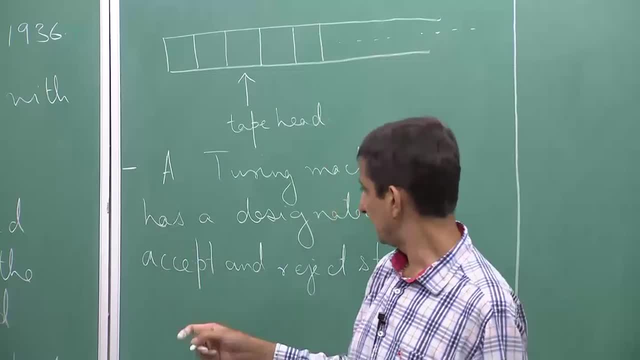 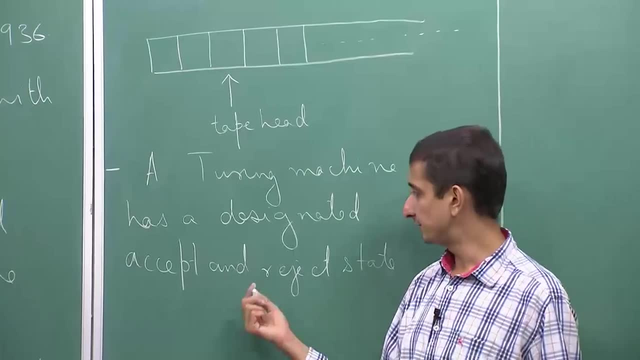 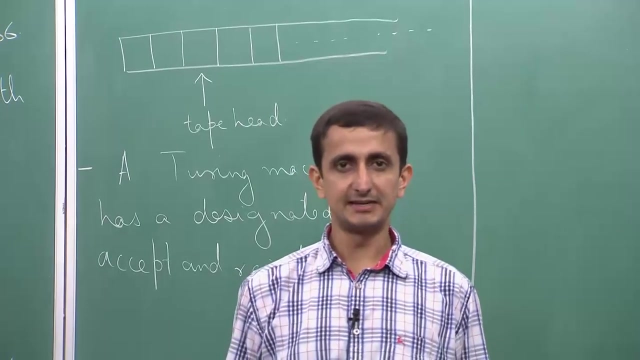 Okay Again, go forward and so on, And the way an input is Okay, Accepted or rejected is basically by means of an accept and reject state. So in the case of a push down automaton, we did not have a reject state. 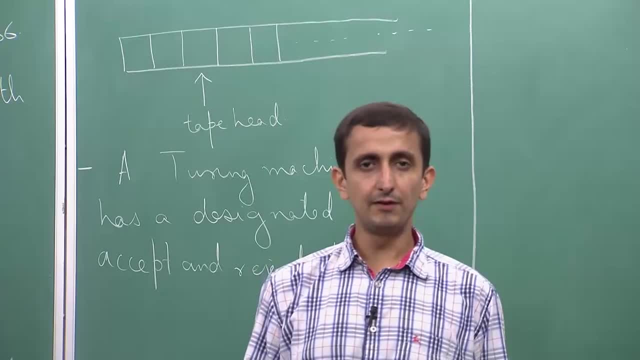 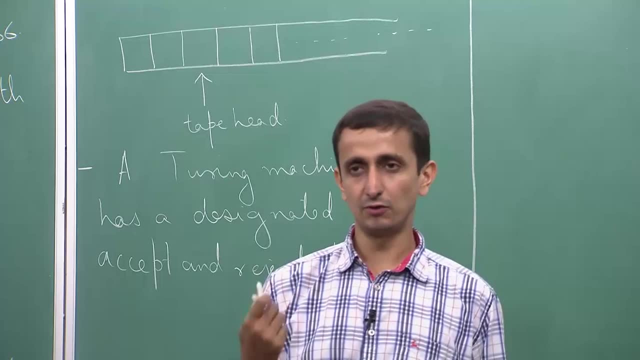 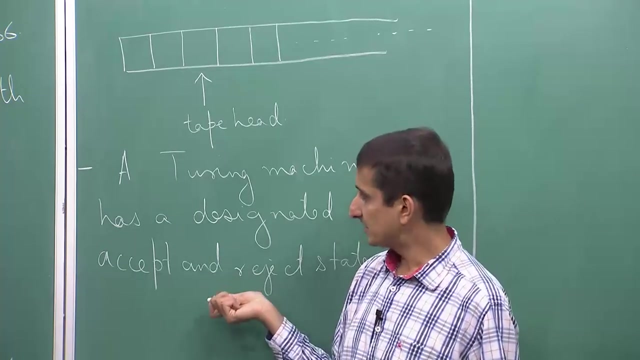 So we said that an input is accepted if the Turing machine is or if the push down automaton is on a accept state when the input is fully read, and otherwise it is rejected. In the case of a Turing machine, As soon as the computation of the Turing machine enters the accept state or the reject state. 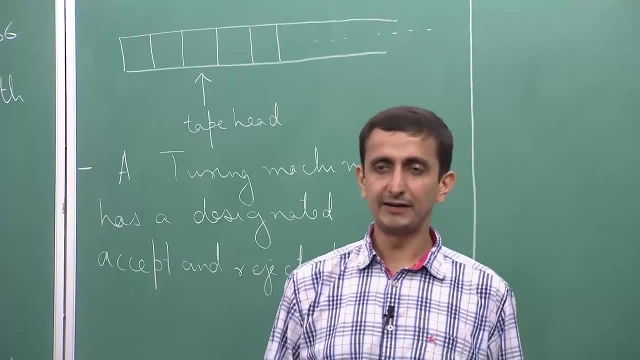 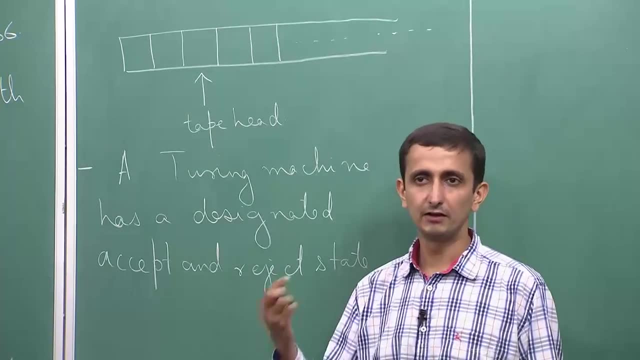 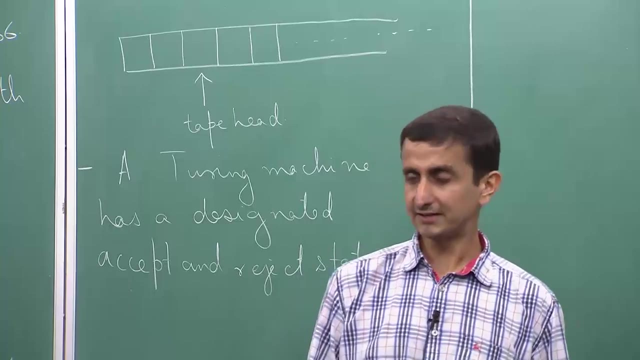 we halt the computation. And if it enters the accept state, we accept the input. If it enters the reject state, we reject the input. Okay, It is not dependent on whether the input is read or not. Okay, The input can be read as many times as necessary. 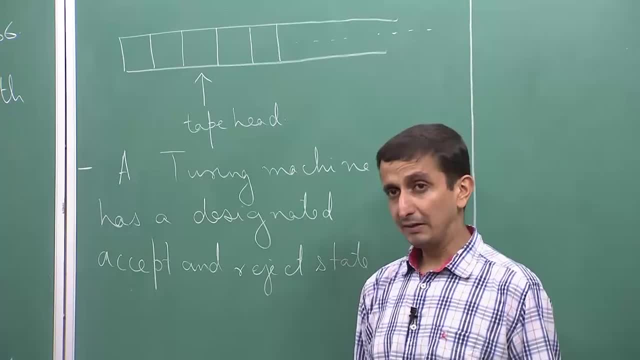 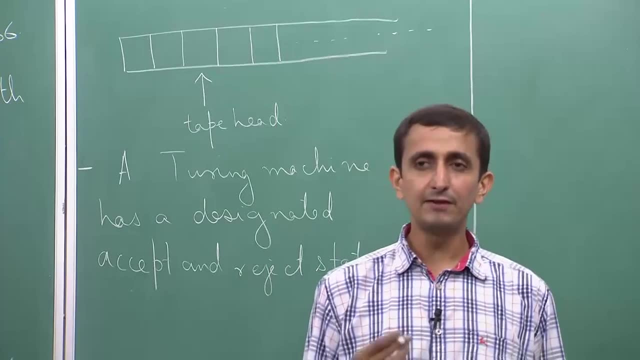 That is point number 1.. And point number 2 is that, Because of this condition that we only halt when we enter the accept or the reject state, it can very well happen that you design a Turing machine which never enters the accept or the reject state. 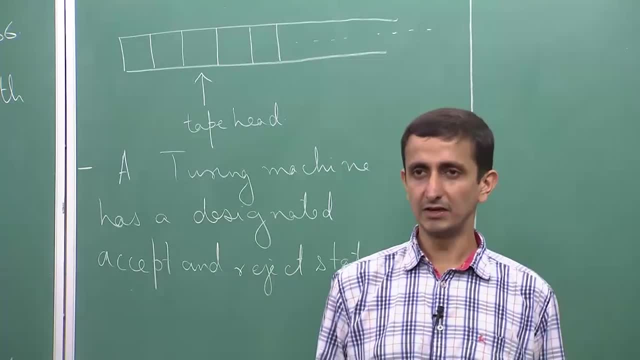 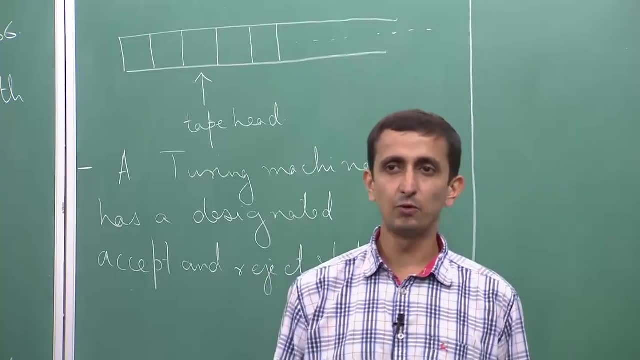 Okay, In that case we say that the Turing machine essentially goes into an infinite loop. It never halts on that particular input. Okay, So you can. for example, you can write programs in C which never halt, Right, You can write loops that run forever. 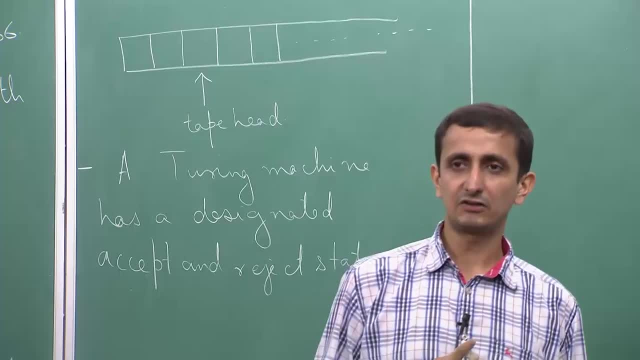 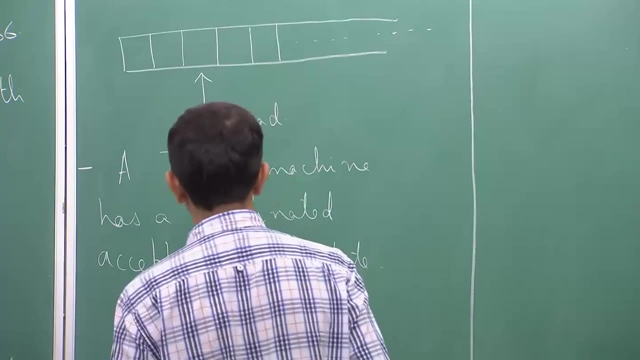 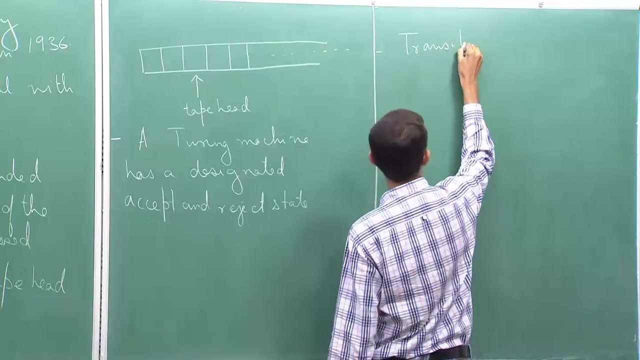 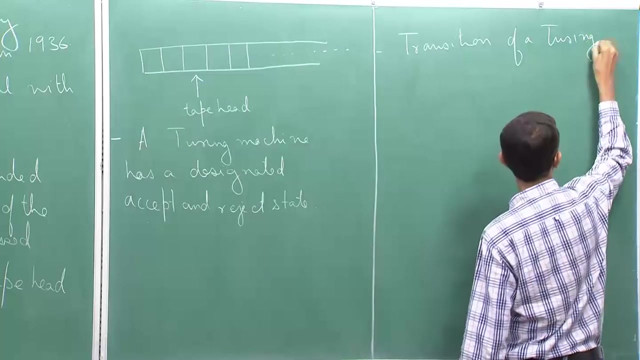 Okay, They never run forever, So similar thing can actually happen with the Turing machine also. Okay, So now how does the transition look like? So, informally, or I want to describe So, transition of a Turing machine essentially looks like this: Okay, 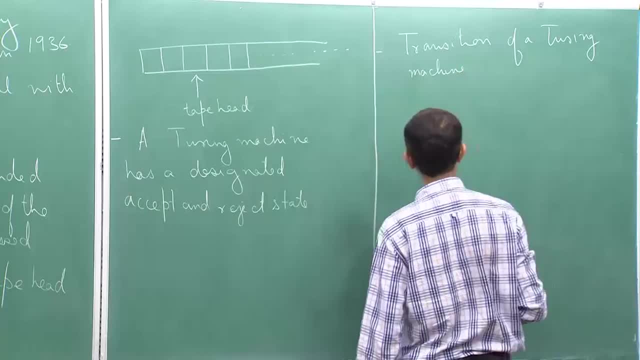 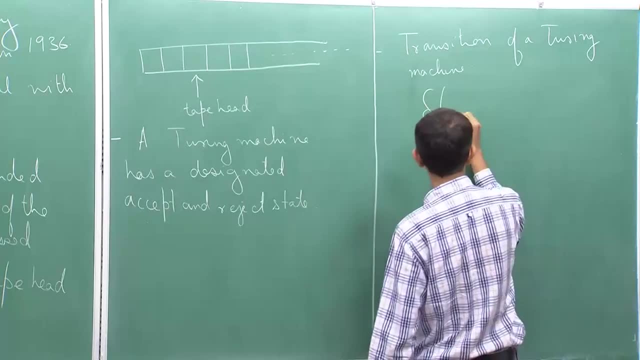 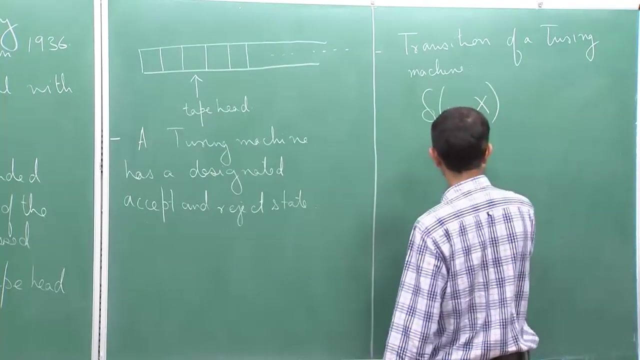 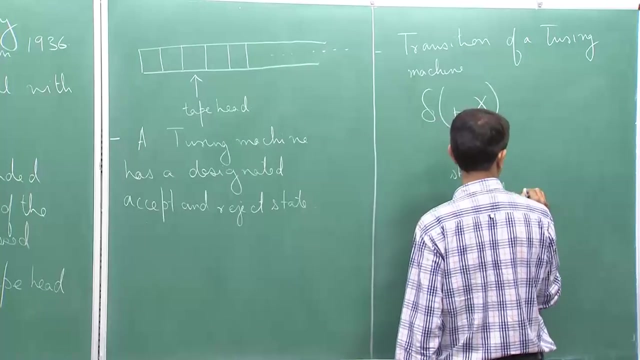 So the transition looks like this: Okay, Okay, Okay. So the transition looks like the following: So we have a transition function, delta, which takes two things: a state p and a tape symbol x. Okay, So this is a state, This is a tape symbol. 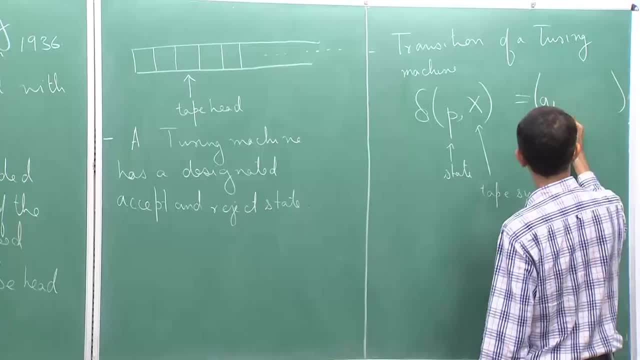 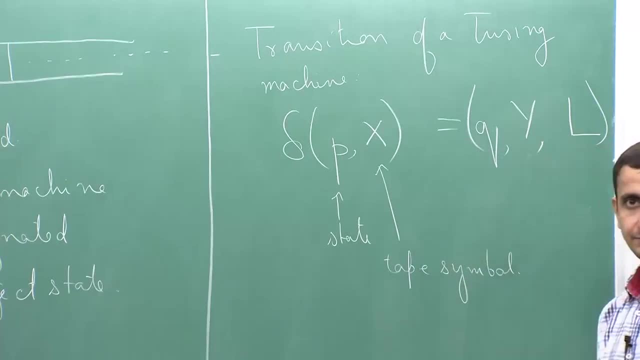 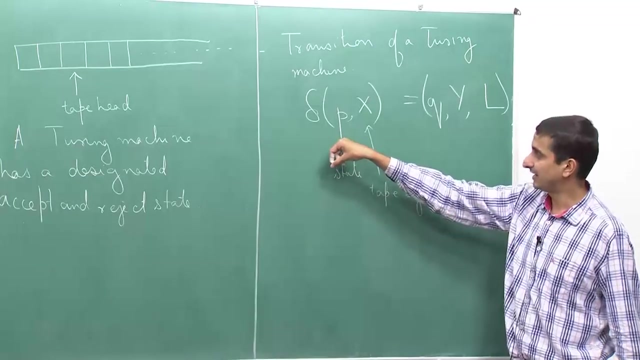 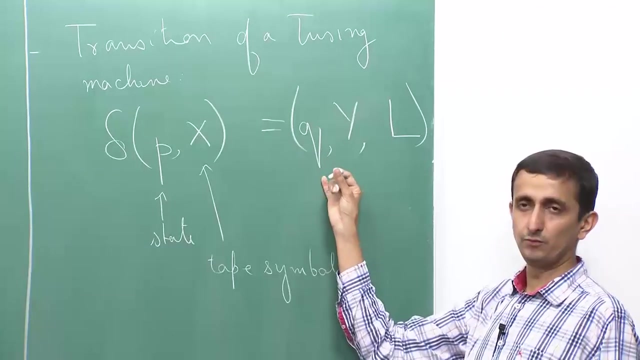 And it produces a triplet: q, y, Okay, Okay. So what are these three things? So, on reading state p from state p, on reading the tape, symbol x. this transition means that the machine goes to state q. It replaces x with the symbol y. 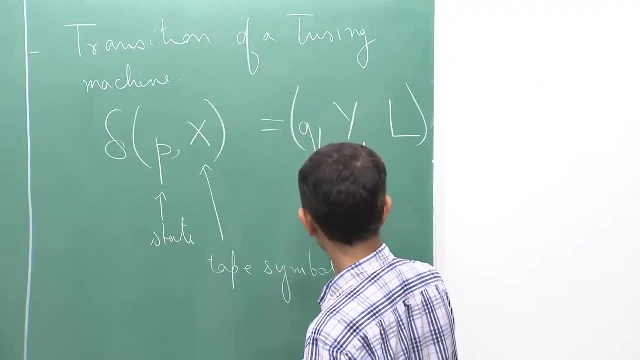 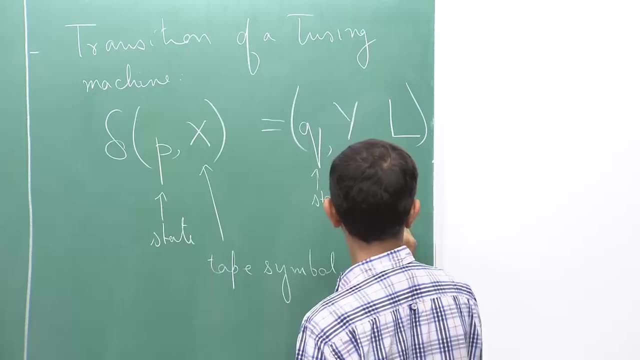 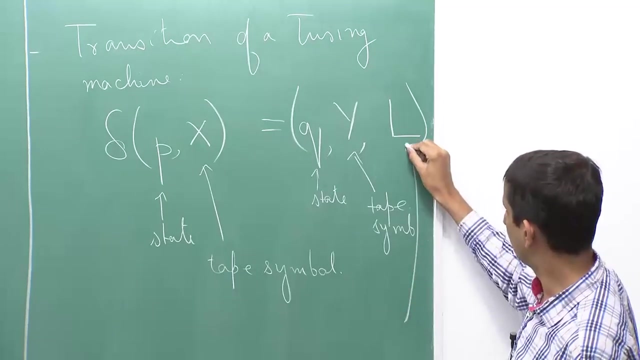 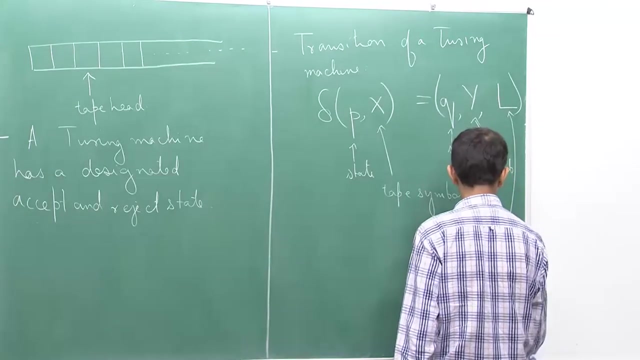 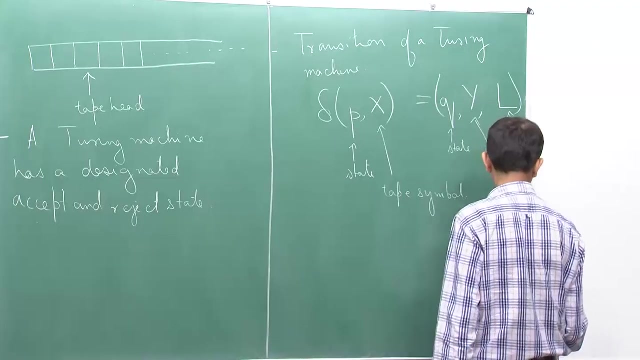 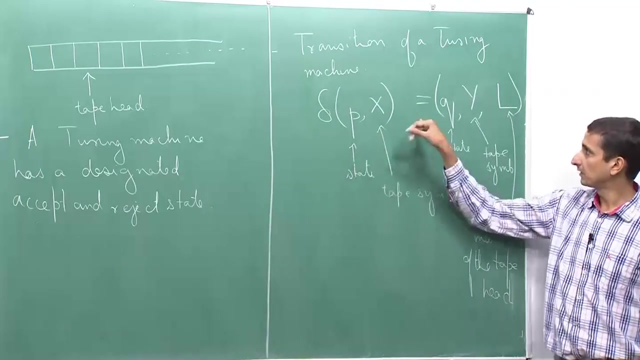 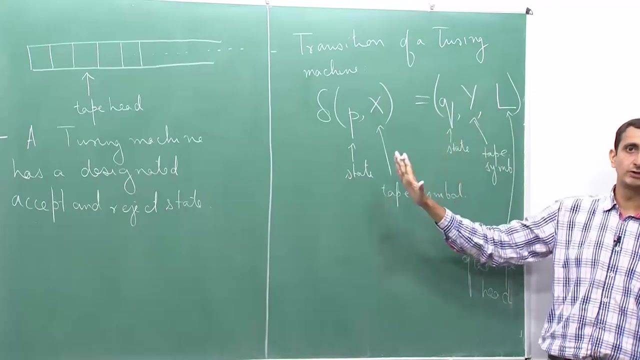 Okay, So this is also a state. Okay, So this is also a state. Okay, So what is the state? So this is a state. This is another T tape symbol. Okay, Here is. So, after reading the symbol x, the machine replaces x with y and the head moves one cell. 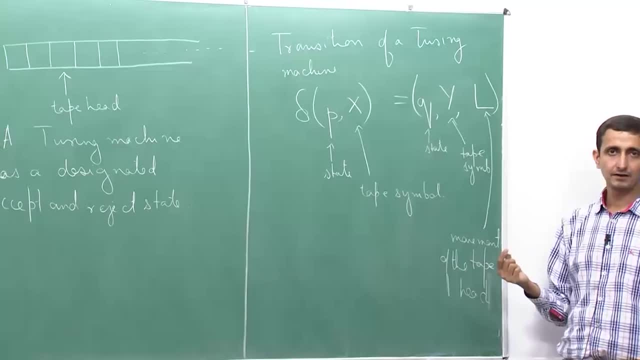 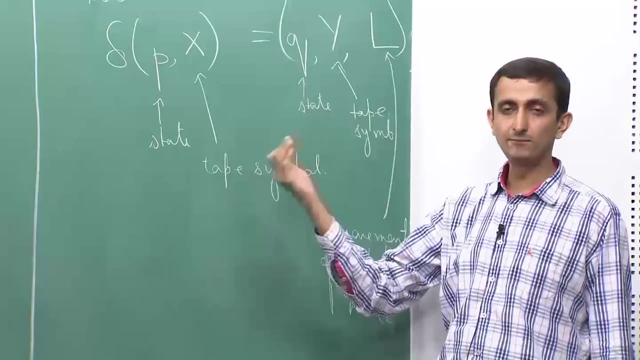 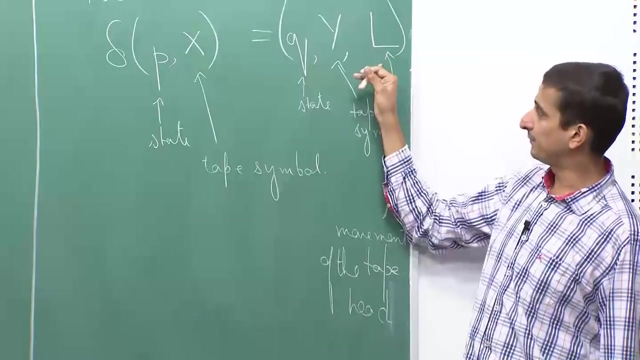 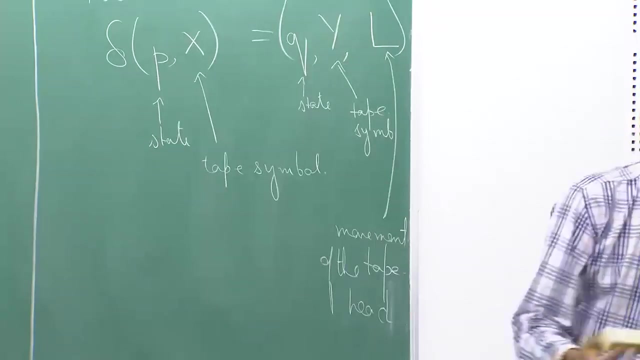 to the left. So instead of l you can also have r, which would mean that the head moves one cell to the right. So I had said earlier that the head only moves either one cell to the left or one cell to the right. So this last parameter, this last element of the tuple, essentially represents that fact. 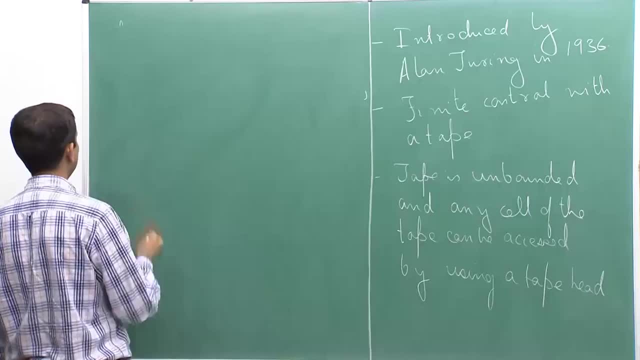 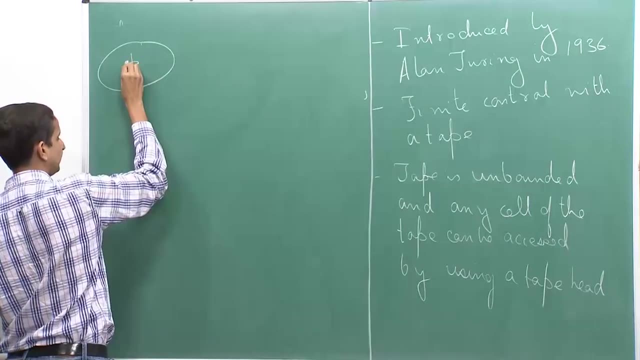 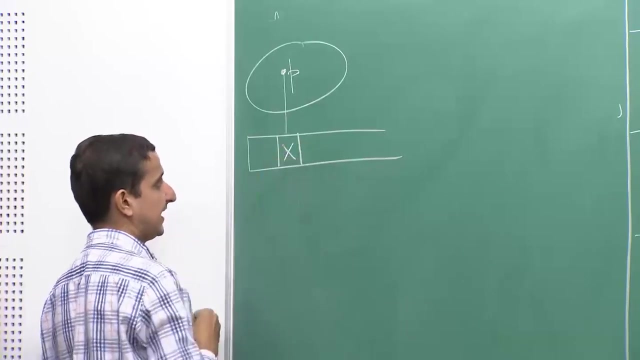 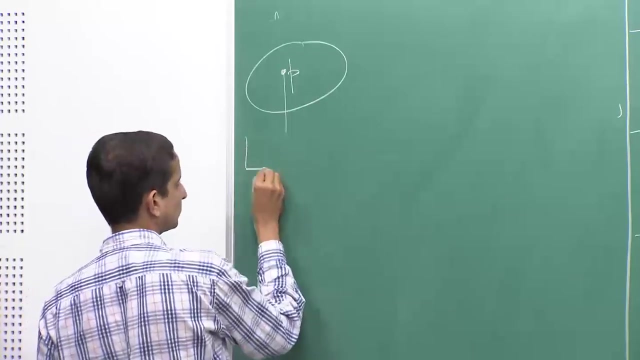 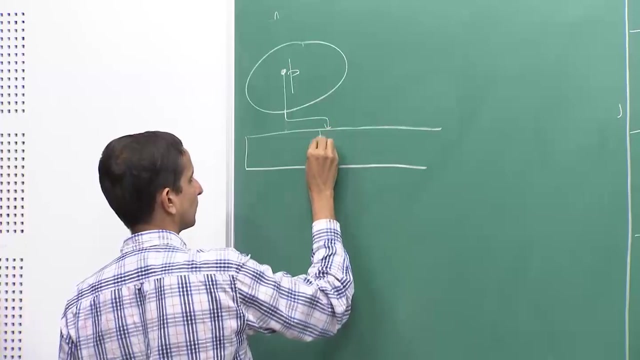 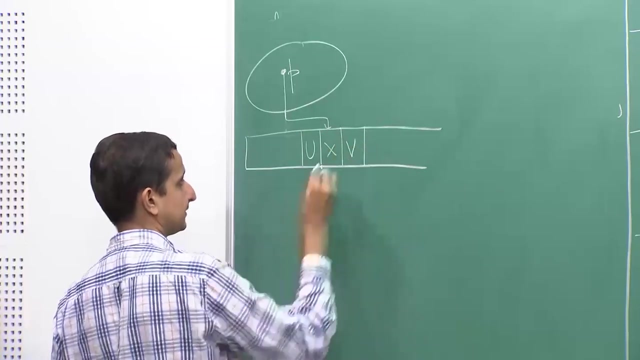 So pictorially, if I want to represent this. so let us say that I have my finite control. the machine is at state p, and here is my tip, where there is a cell with x written on it, And maybe there is. so let us say, the left cell has u written on it, the right cell has 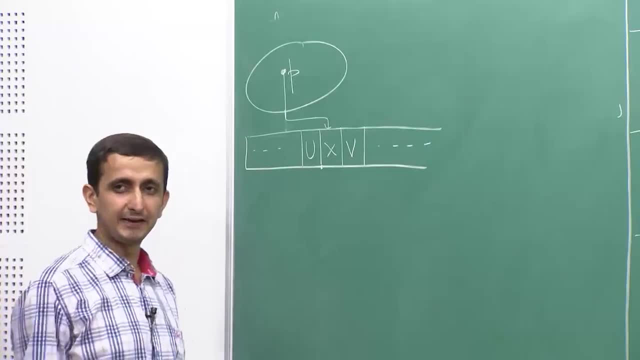 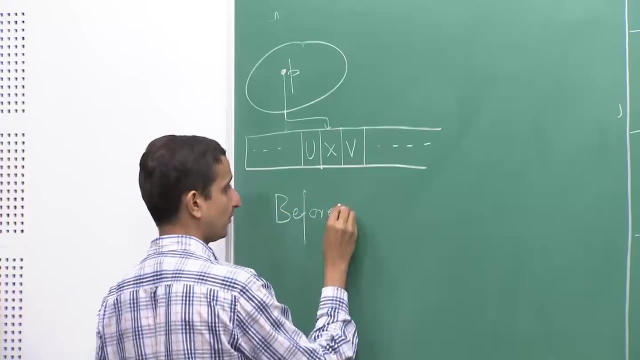 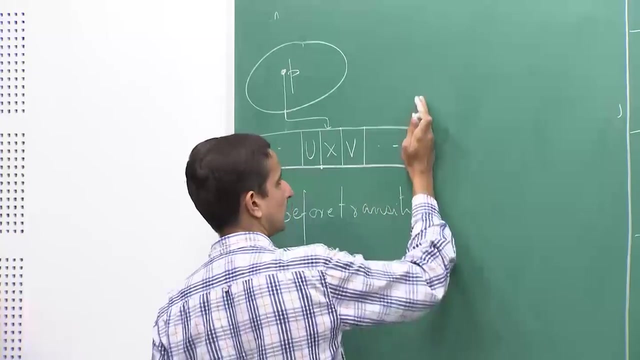 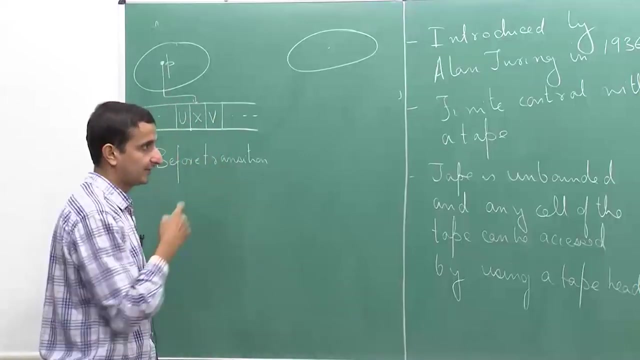 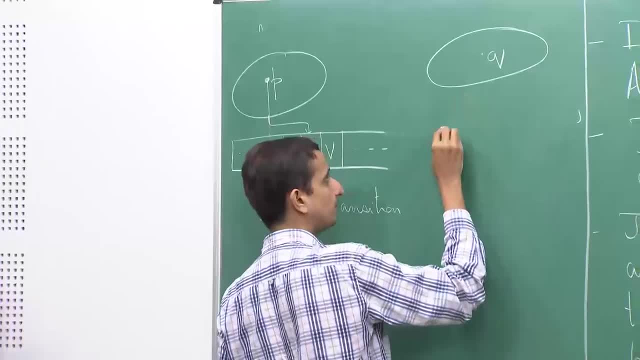 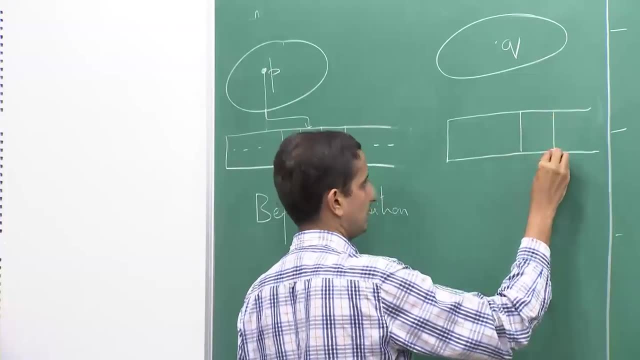 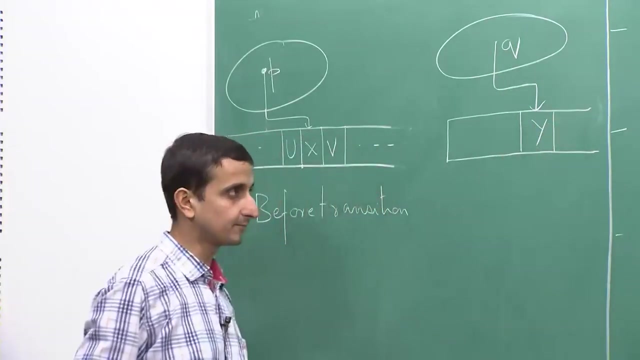 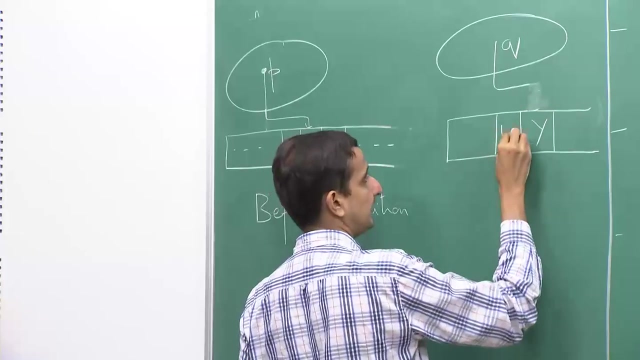 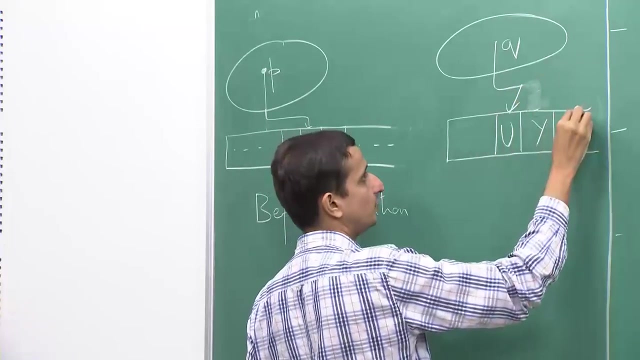 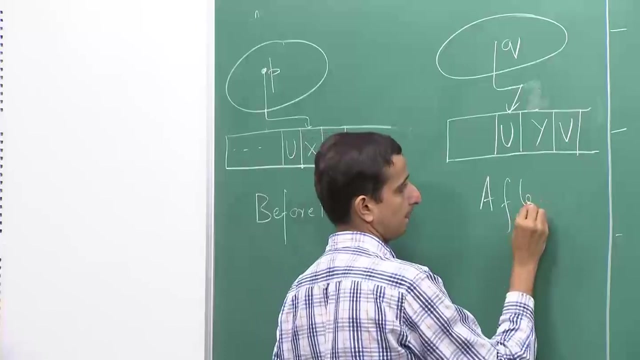 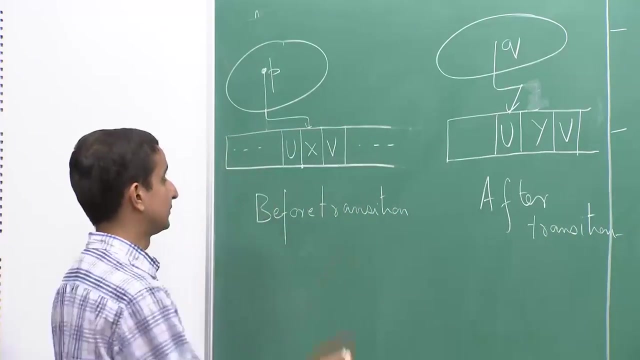 So after the transition it moves to state q on my tape. I replace x with y and the tape head moves left. so the tape head will basically point to u. now, okay, So this is basically after the transition. so if I denote the transition, 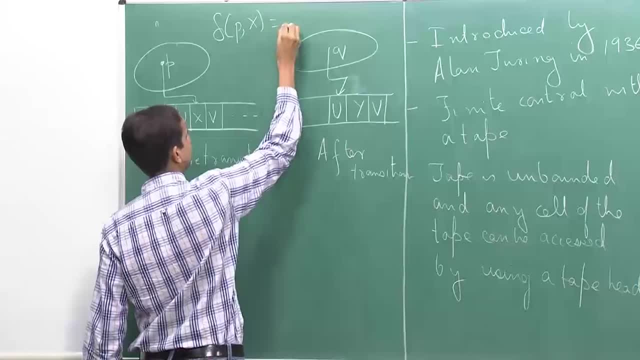 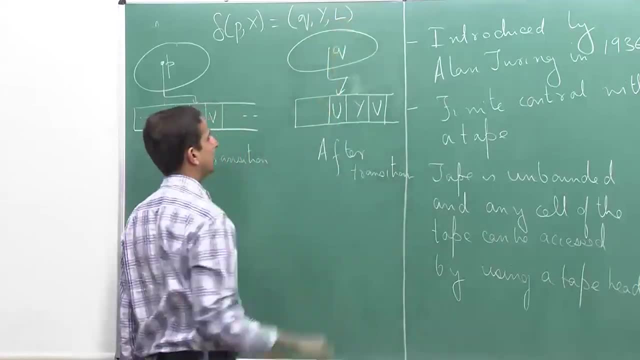 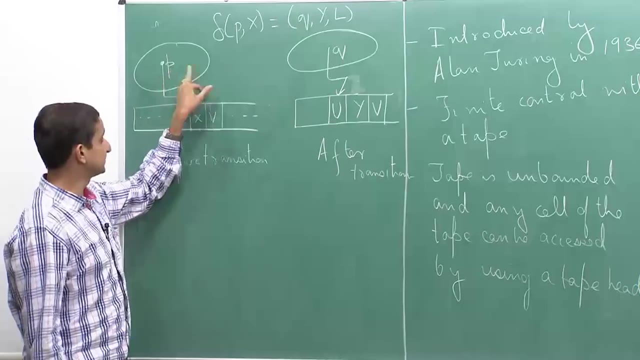 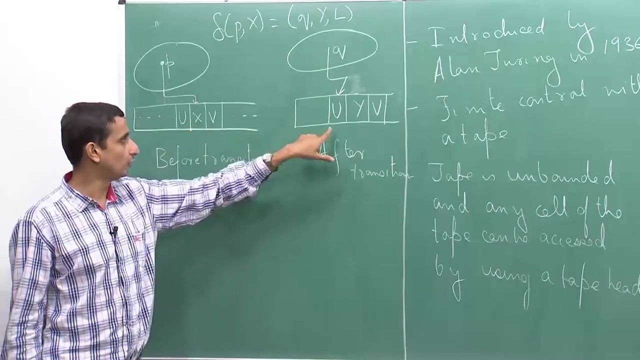 as delta px equal to q, y, l. okay, So on reading x, it replaces x with y, it goes from state p to state q and the tape head it moves from the cell which it is currently pointing to to the cell left of it. So this: 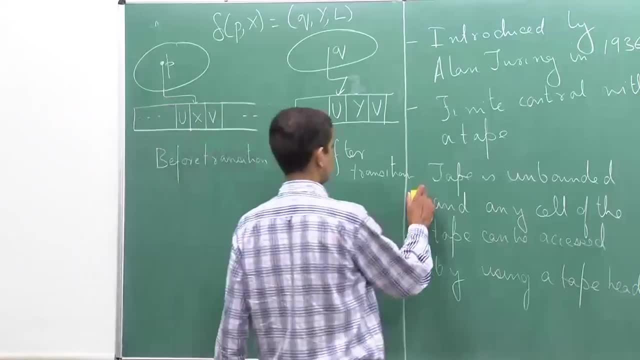 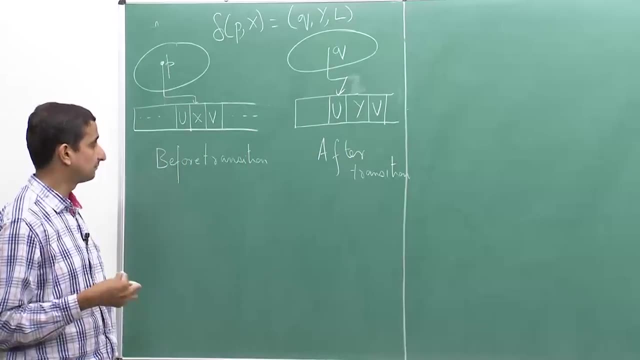 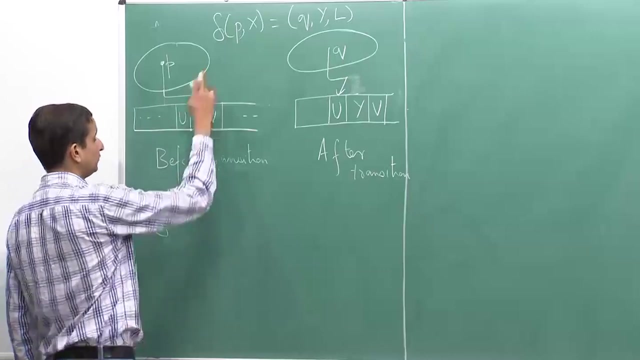 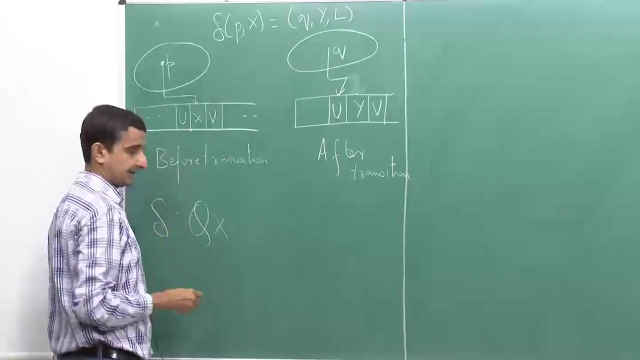 is each transition. So therefore, if I want to formalize this, what does the transition function? I mean how to define the transition function. So the transition function delta is essentially a function which takes two arguments. So first it takes a state, then it takes a tape symbol. So let's say I represent the tape symbol. 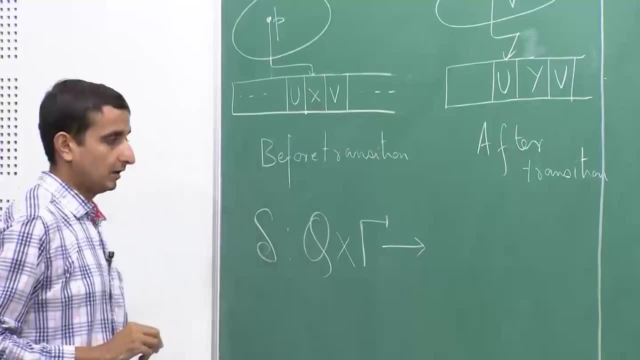 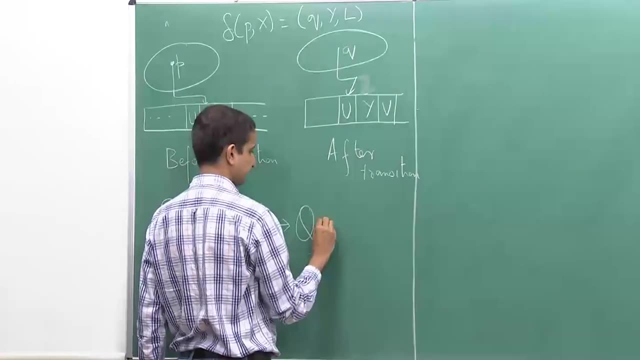 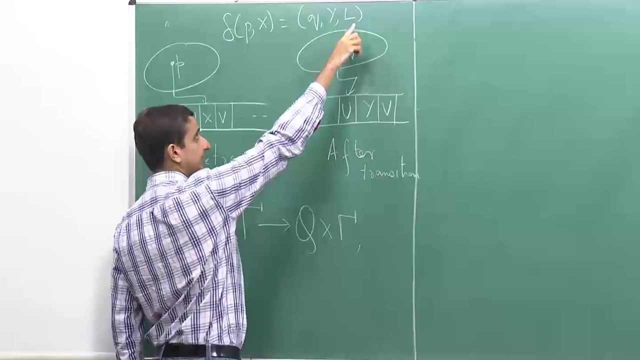 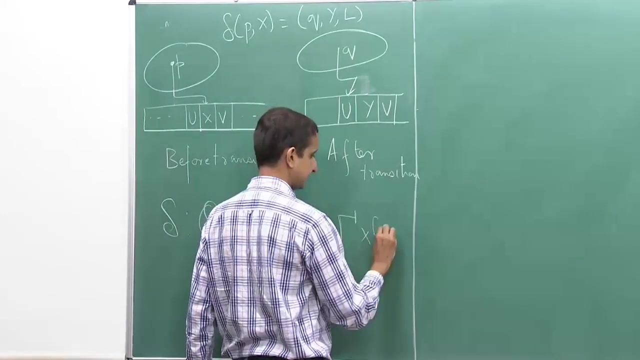 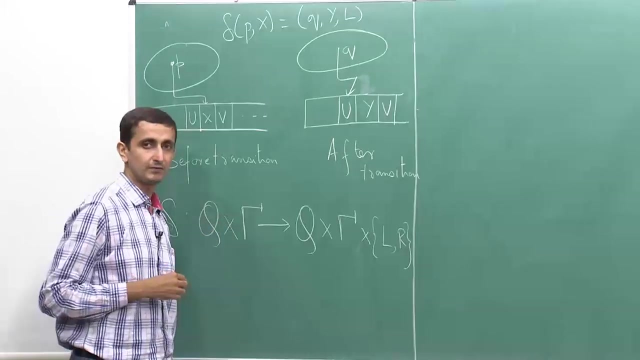 with gamma. okay, Then it produces a triplet, so it produces a state, a symbol y. Now let's, and it gives us a bit which tells us whether to go left or right, So cross two bits, either left or right. So this is the transition function of a Turing machine. 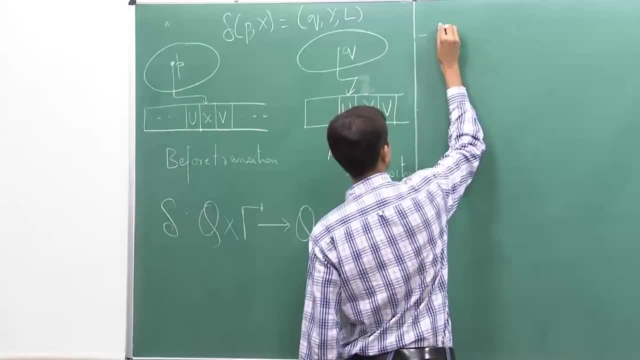 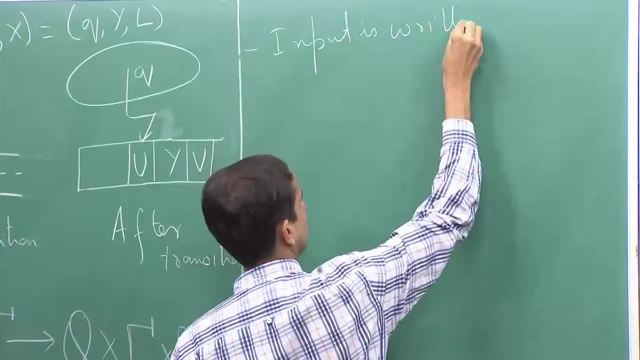 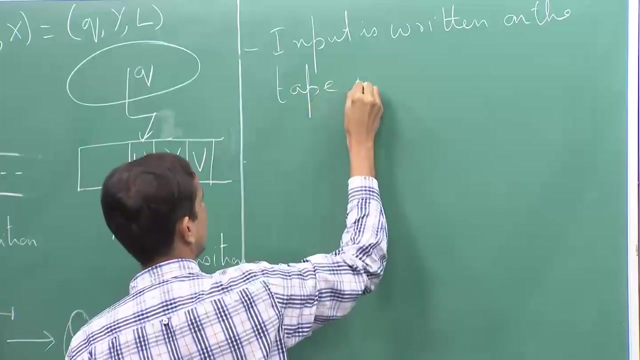 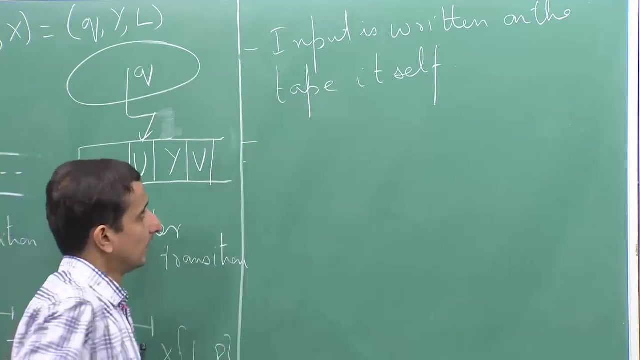 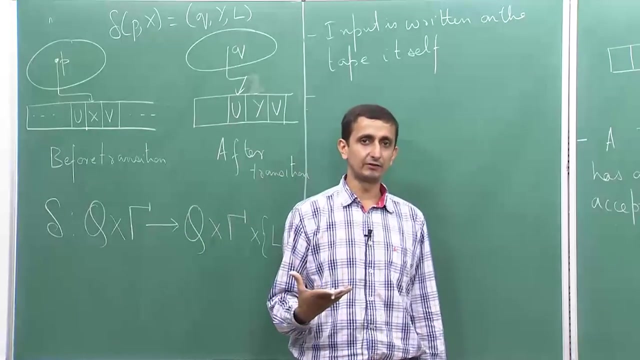 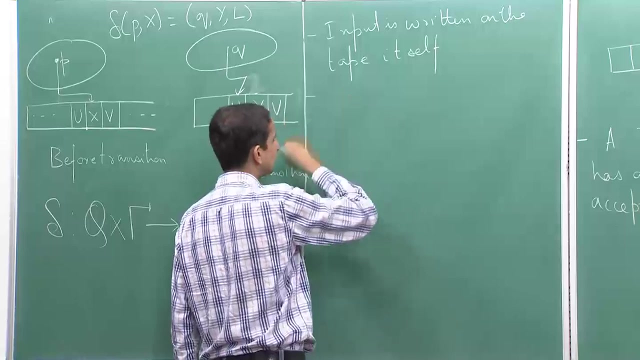 So, as I said, the inputs is written on the tape. so it is written on the tape. I mean, actually, you actually begin the computation with only the input written on the tape and there is a special symbol. So before I say that, so we will assume that. so, because the input is written on the tape, 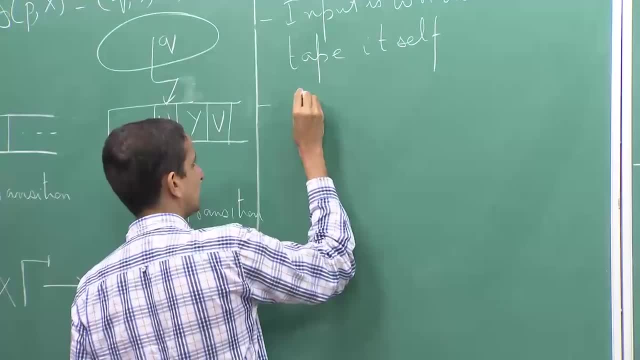 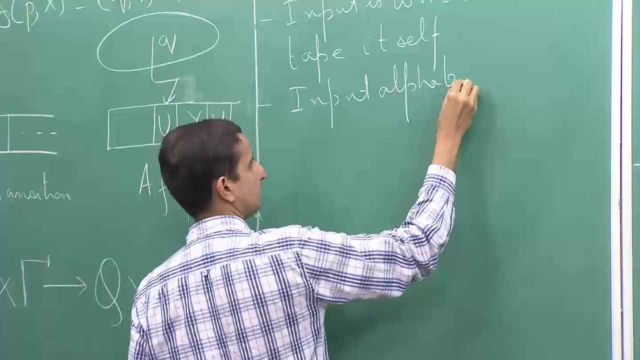 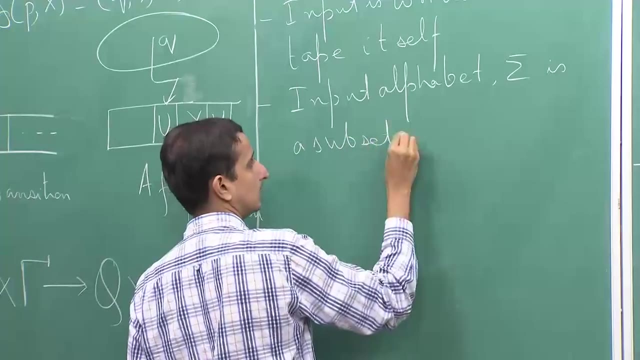 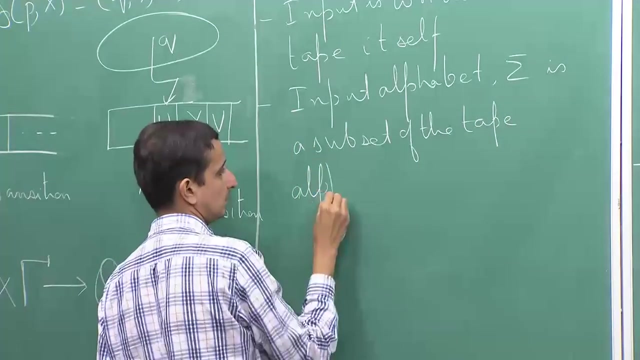 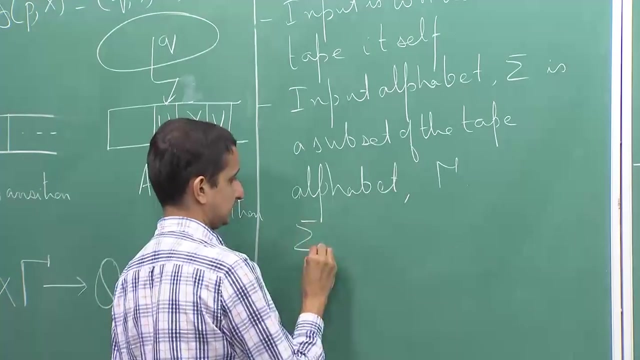 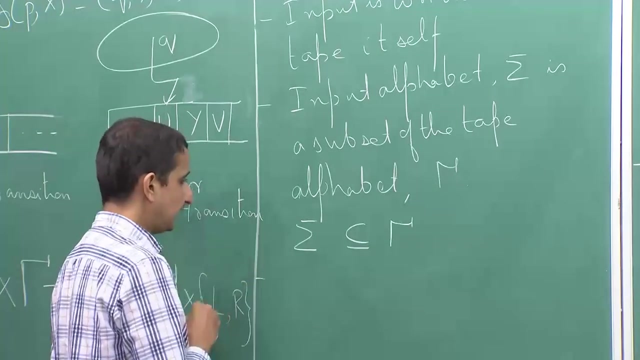 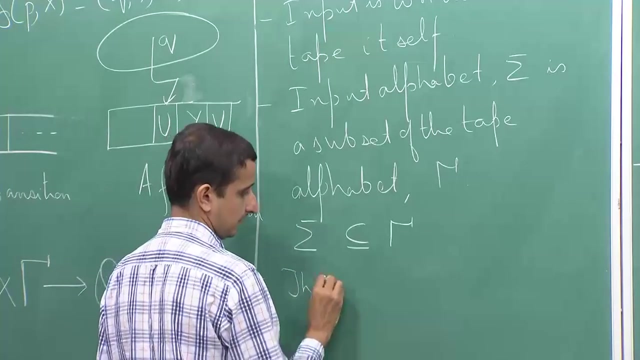 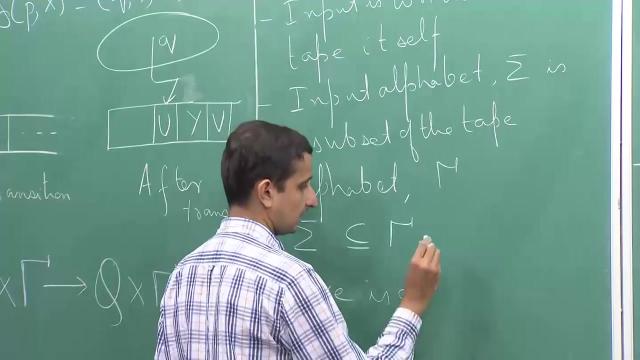 itself. what we will assume is that the input alphabet sigma is a subset of the tape alphabet gamma. Okay, Thank you. So basically, sigma is a subset of gamma And in fact, this is a proper subset, because we will assume that there is a, so there is. 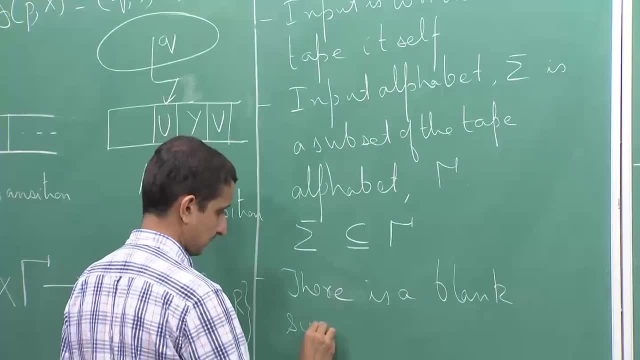 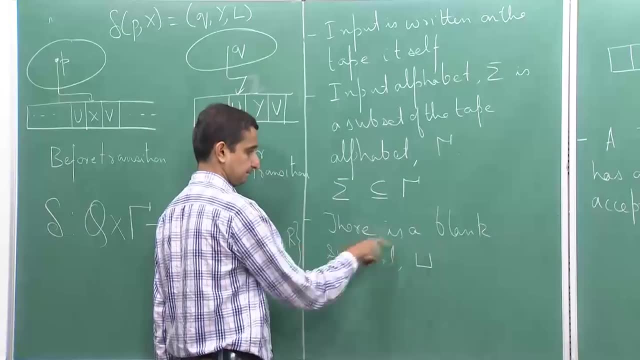 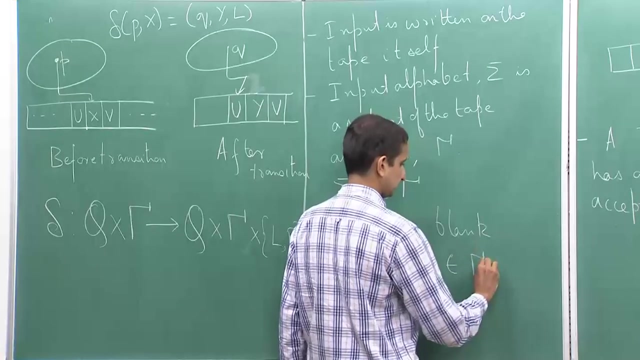 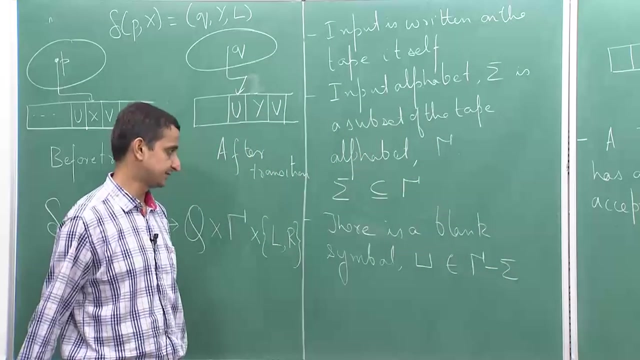 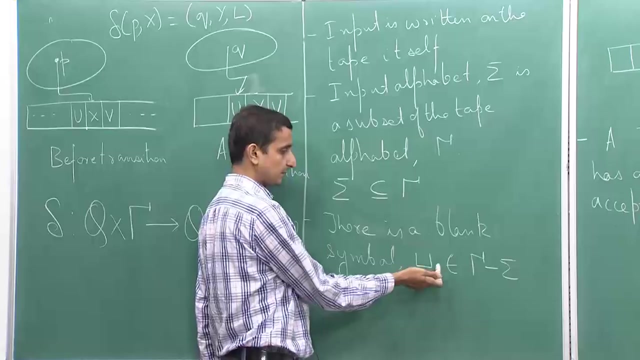 a blank Symbol. Okay, So this is represented as a open box like this, which is, which belongs to the tape: alphabet gamma, but not the input: alphabet sigma. Okay So there is a blank symbol: gamma, which belongs to. sorry, there is a blank symbol which belongs. 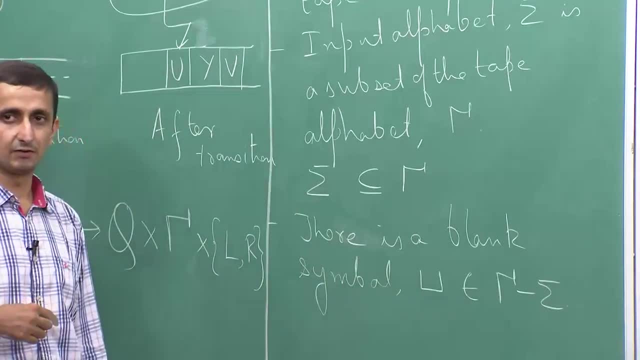 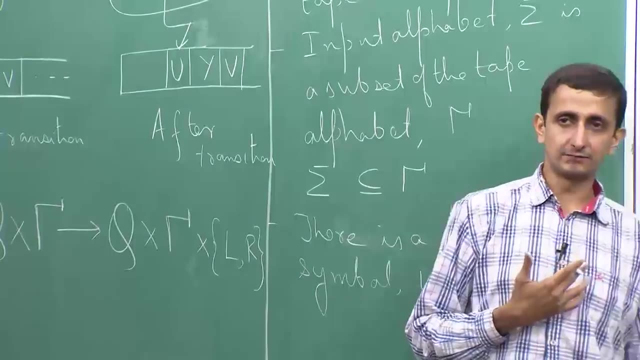 to the tape alphabet sigma. Okay, So there is a blank symbol which belongs to the tape alphabet gamma, but it does not belong to sigma. Okay, So this is just to distinguish the input from the remaining contents of the cell. Okay, 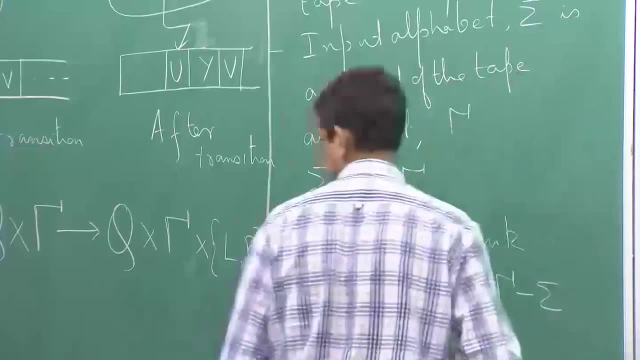 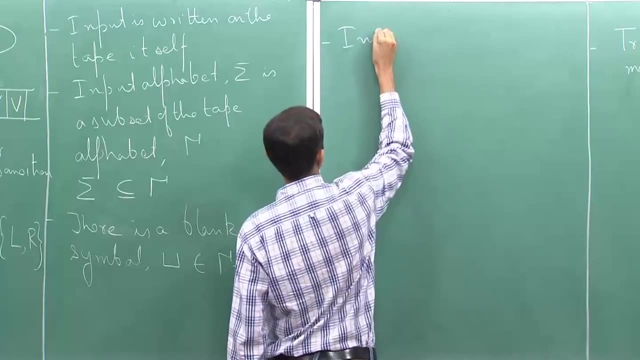 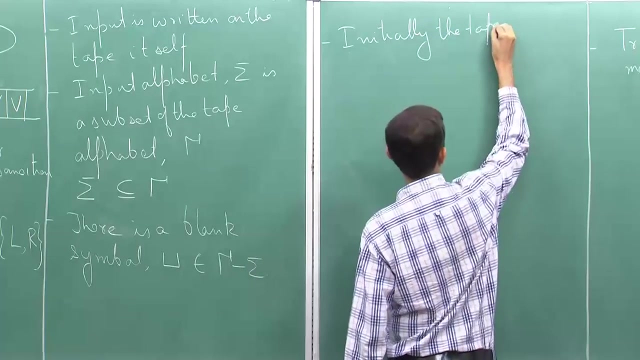 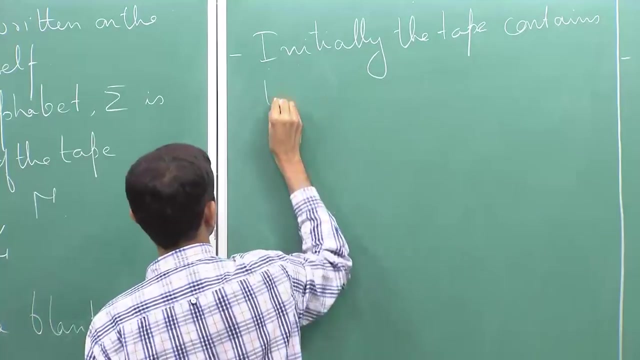 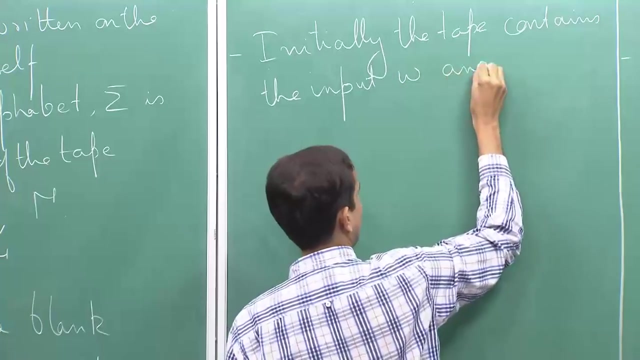 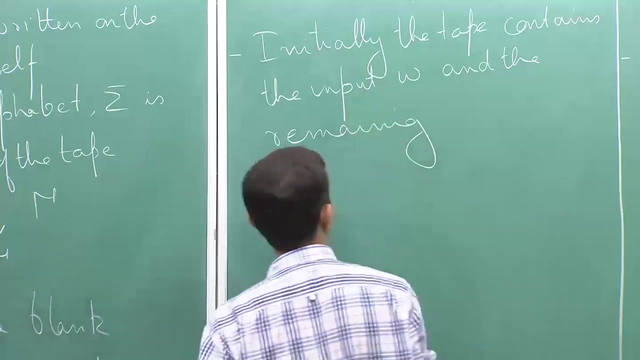 So at the very beginning, what we will assume is that. so in the beginning, we will assume that. so initially, the tape is written on the tape: alphabet: sigma: Okay, Okay. So the tape contains the input w and the remaining cells. 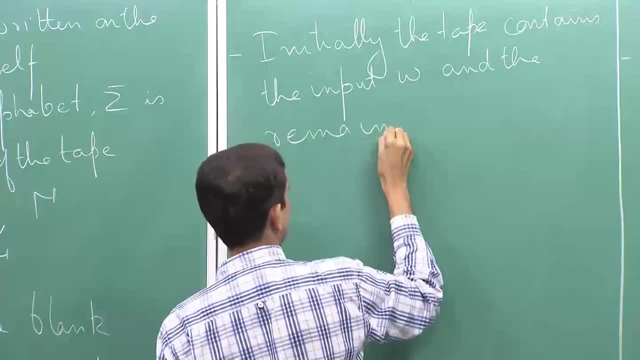 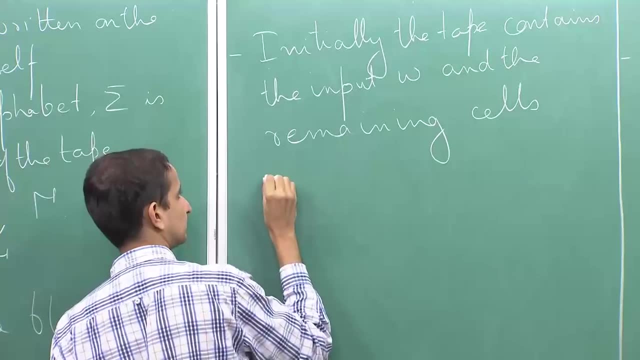 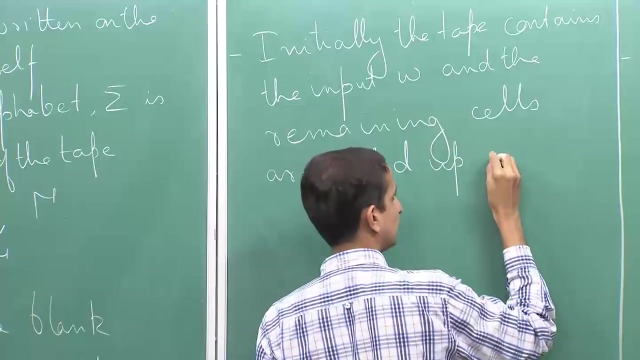 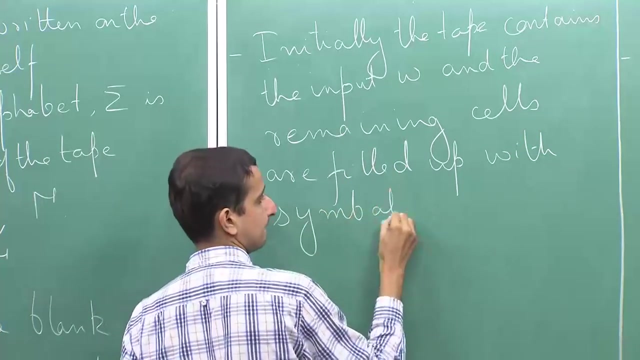 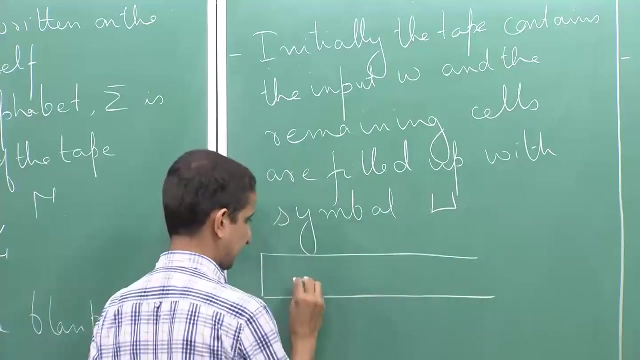 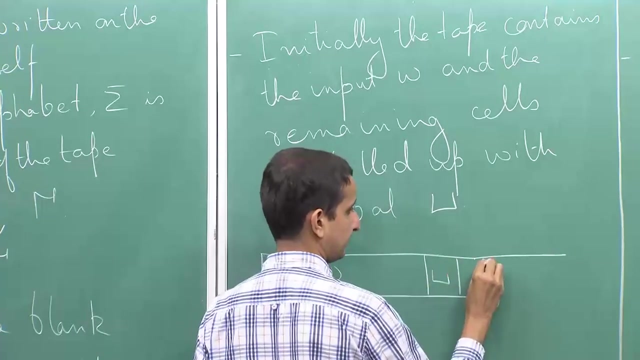 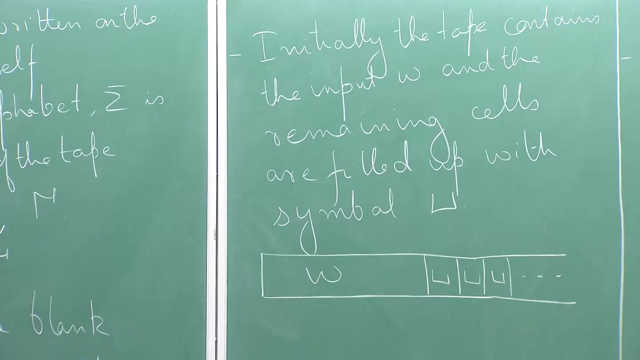 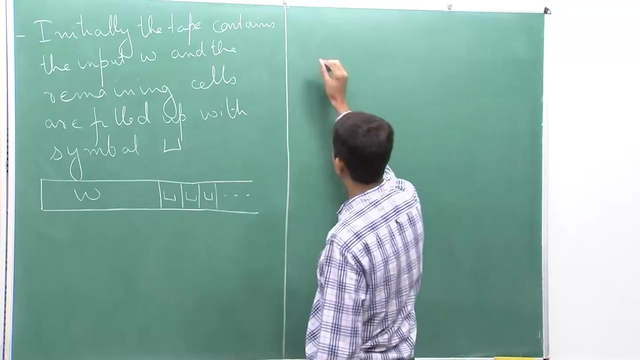 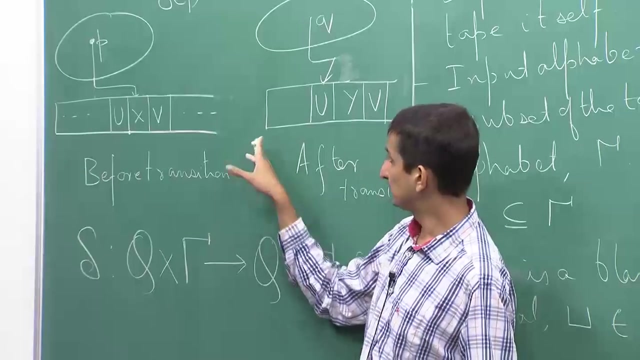 Okay, Okay, Okay, cells are filled up with the symbol. so initially, basically, we have the tape which contains W till let us say some point, and the remaining cells are filled up with blank. so this is the initial configuration. So one more point. so, because we have this assumption, that, or because, if the way we define, 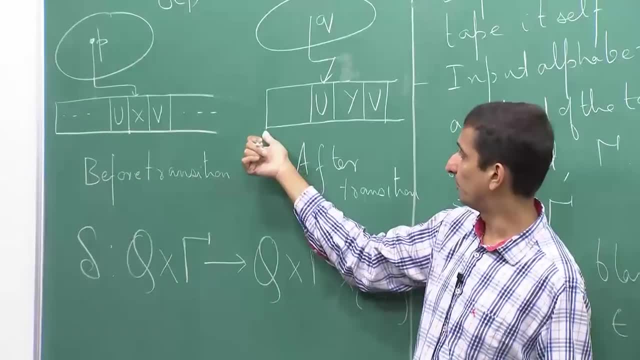 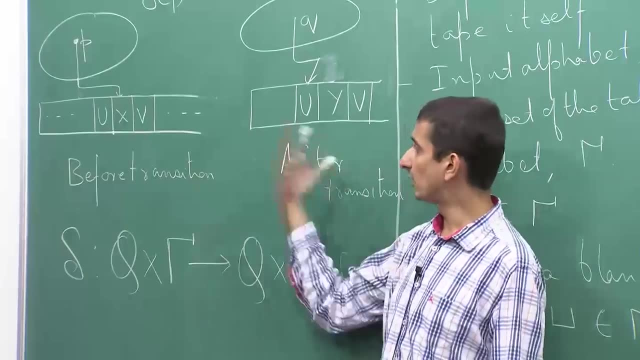 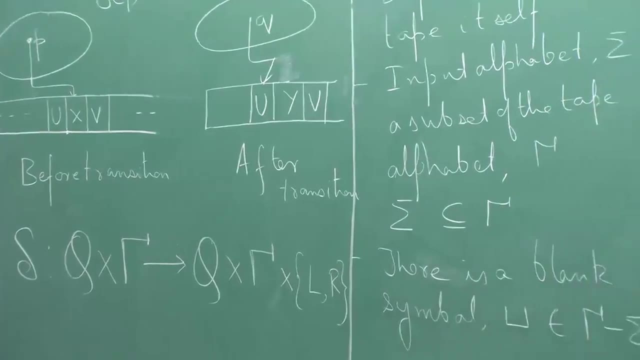 a tape. So the tape is bounded on one side. so when we look at the tape, if I look at the left most cell of the tape, I cannot go beyond the left most cell. I cannot go to the left of the left most cell. so therefore, when I define the transition function, I need to 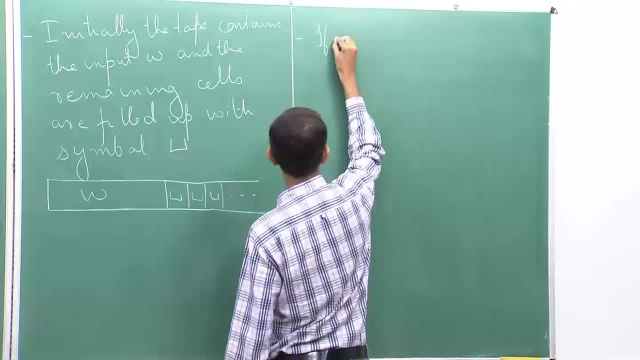 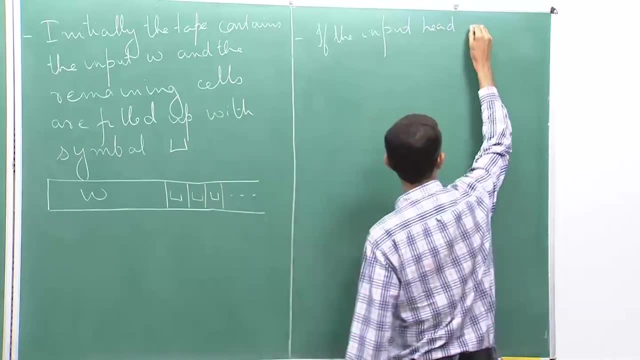 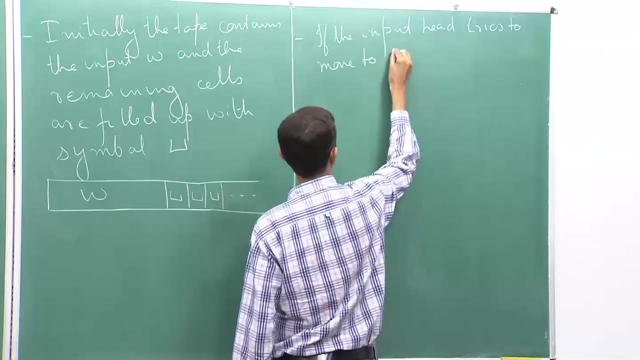 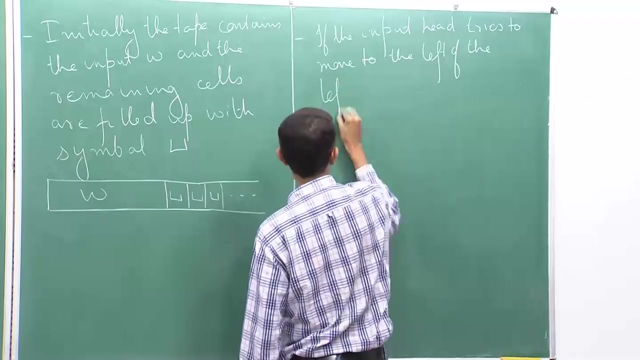 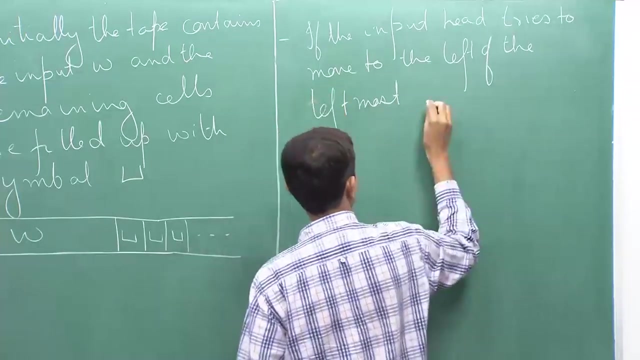 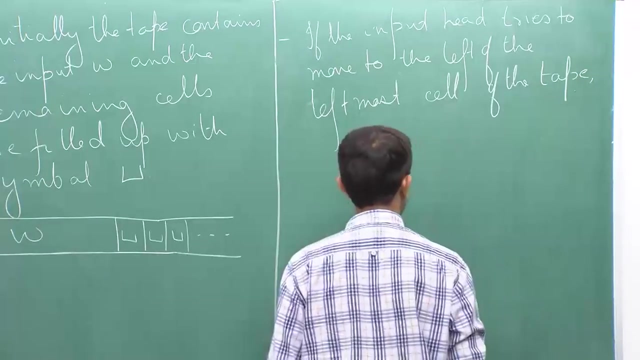 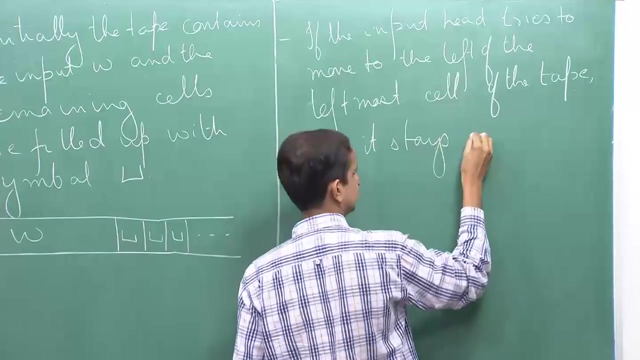 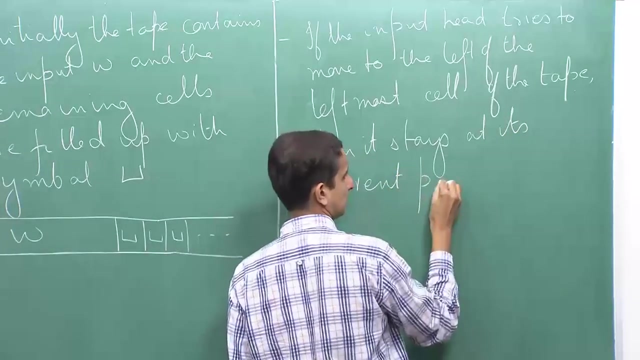 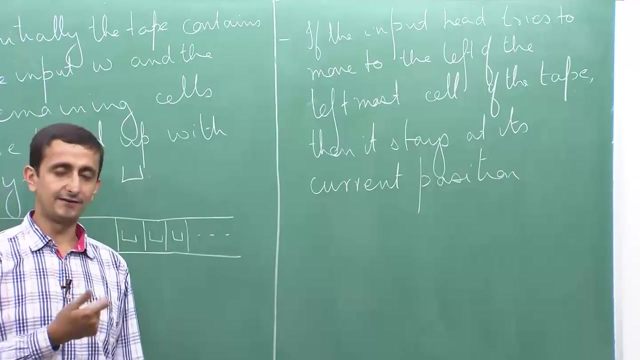 have this additional point that if the input head tries to move to the left of the left most cell of the tape, then it will not go beyond the left most cell. Okay, Okay, Okay. So if the input cell stays at its current position, so if the input cell actually tries, 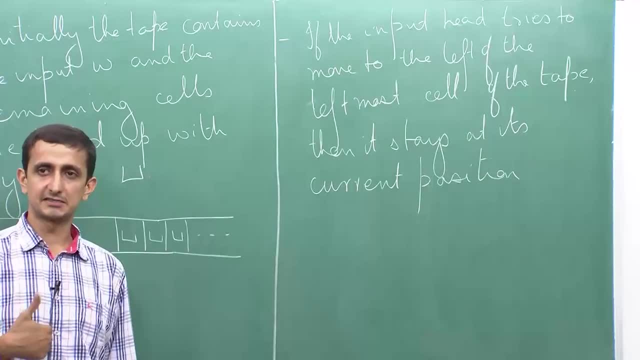 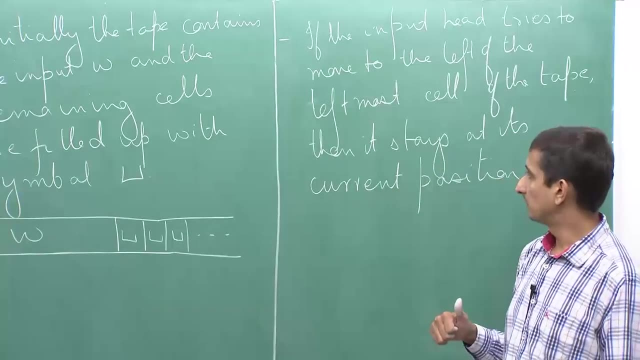 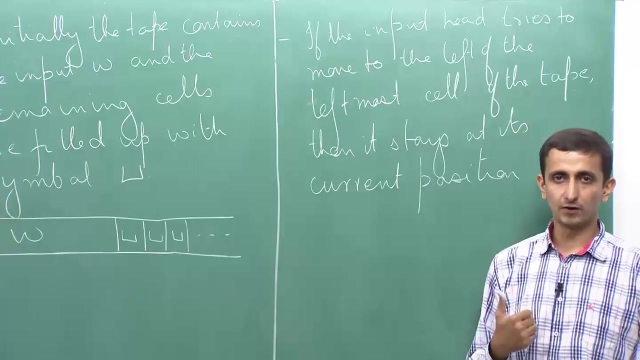 to move to the left, then it will not make that move and basically just stay at its current position. Okay, So this is what we need, Okay, Okay, So we need to make this assumption about the transition function in order for it to 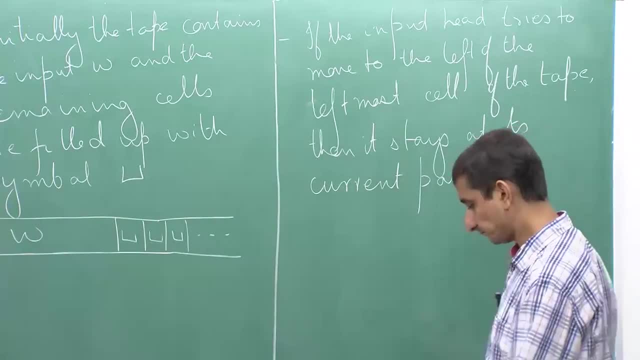 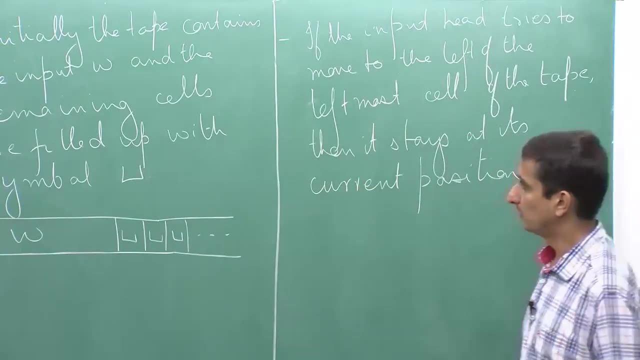 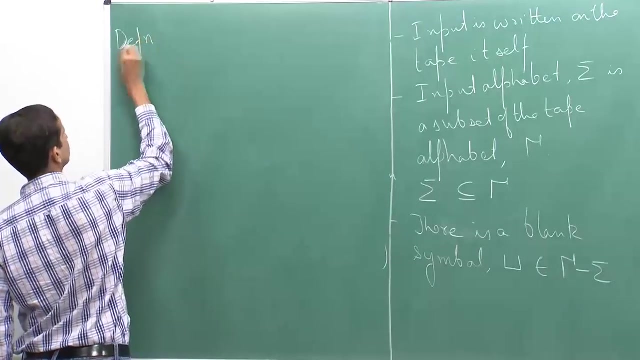 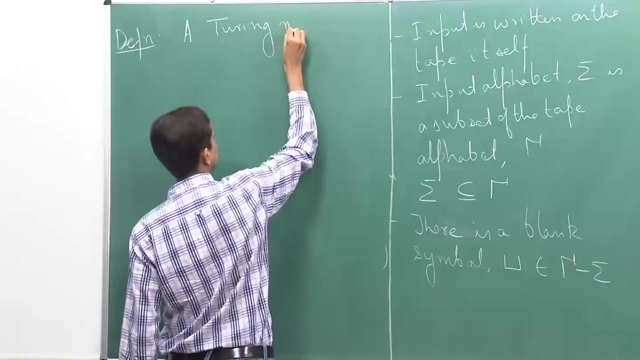 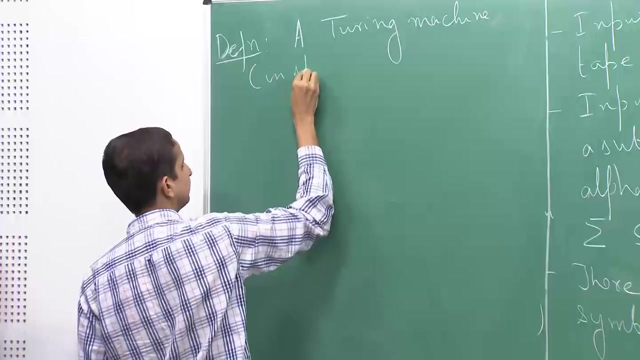 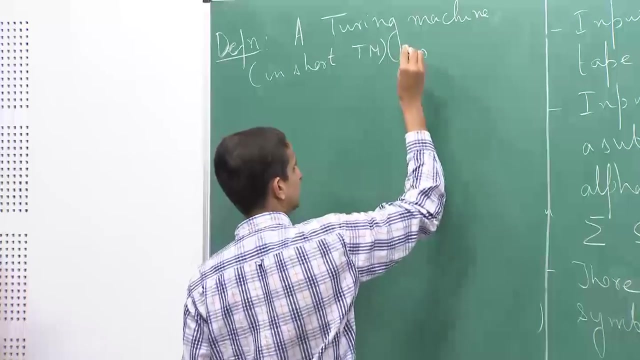 be a complete function. So now that we have all these points, now we can give the formal definition of what a Turing machine is. Turing machine, in short, Tm is the tuple. let us say m equals q. let us say q is the. 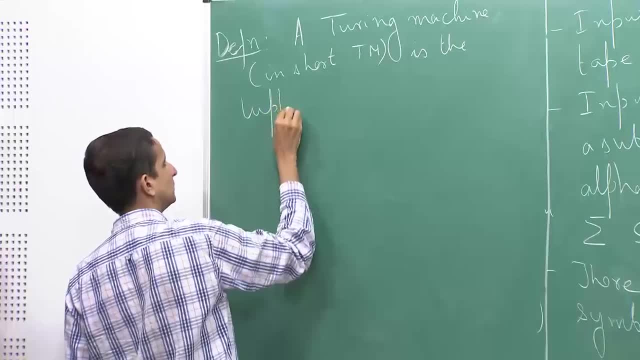 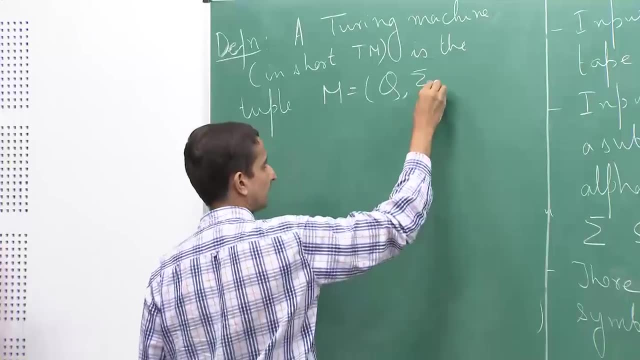 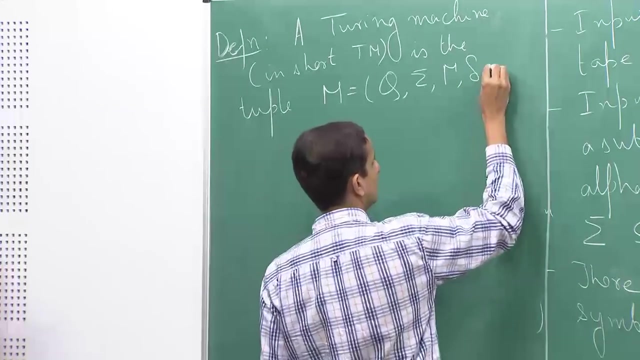 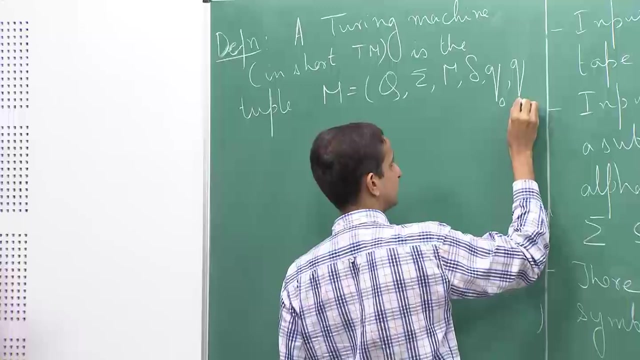 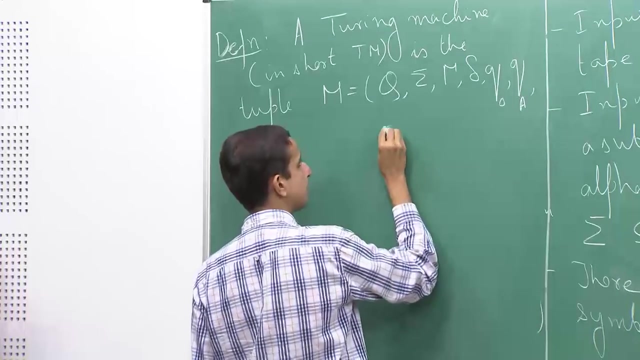 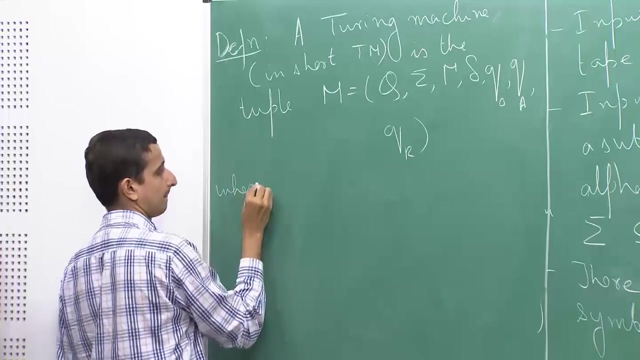 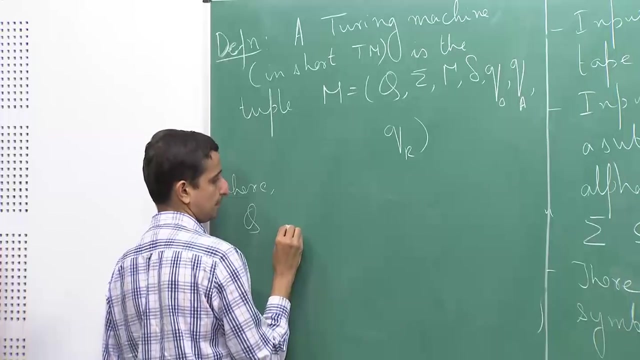 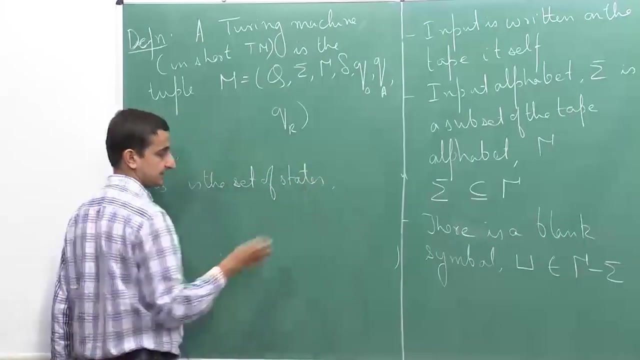 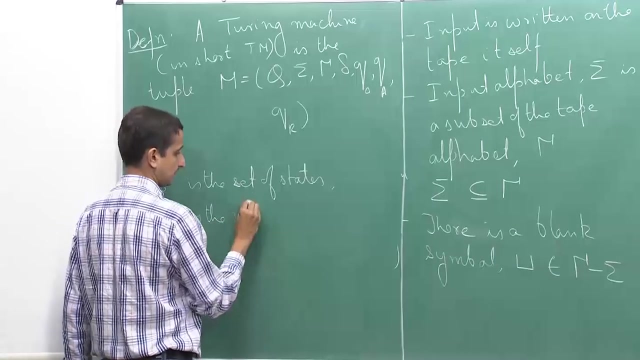 tuple, Okay, Okay, Okay, Okay, Okay, Okay. So we have q, sigma, gamma, delta, q naught, This is the start state, and we have two other states: q, a comma, q, r. Okay, Where, Here, Of course, Q is the set of states, sigma is the input. 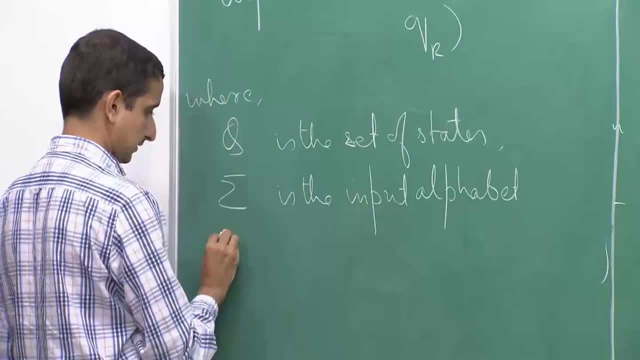 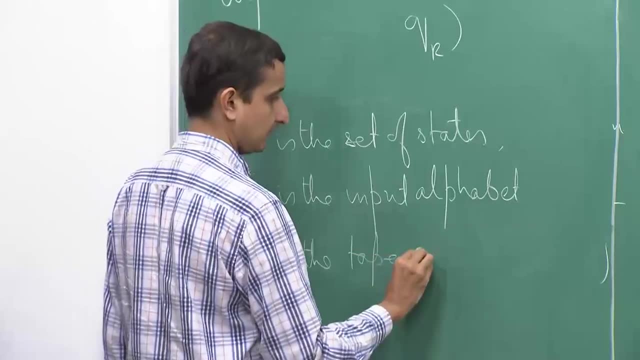 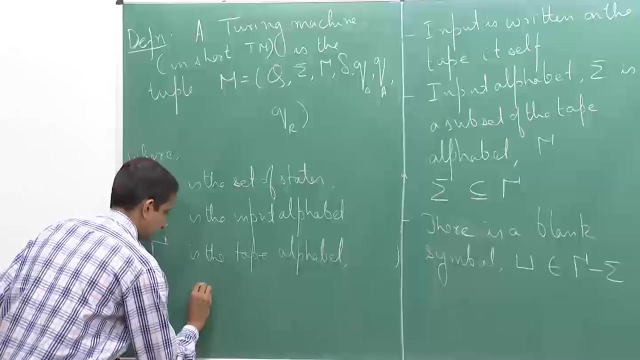 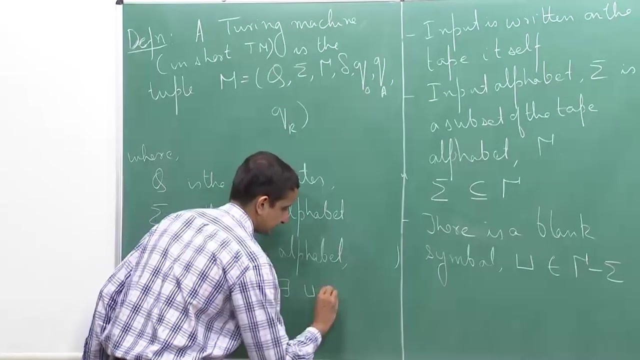 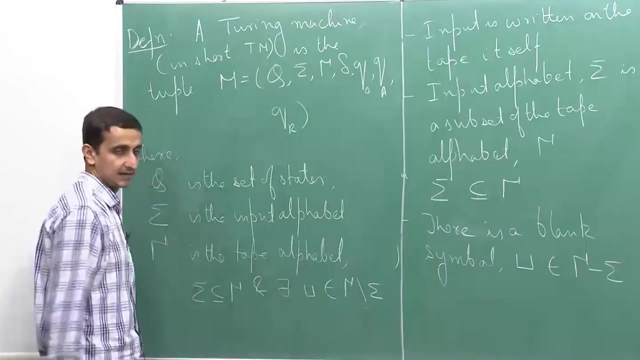 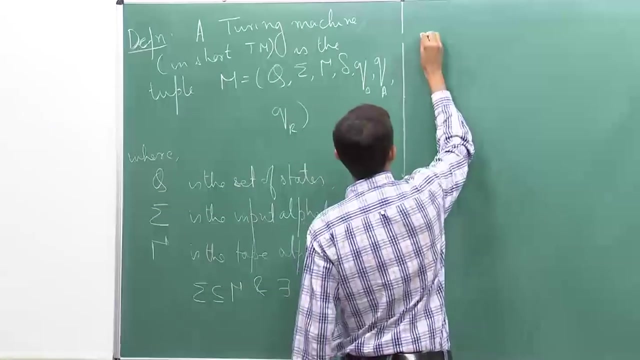 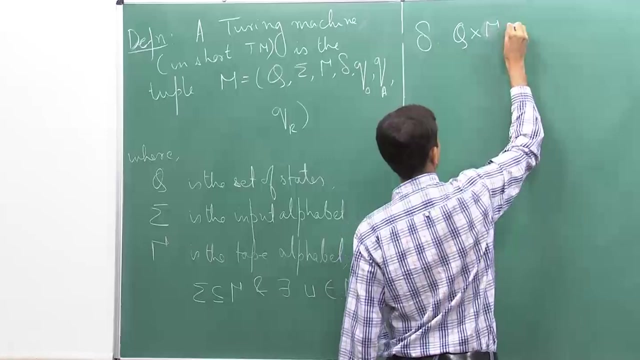 alphabet gamma is the tape alphabet, where sigma is a subset of gamma and there exist a blank symbol which is contained in gamma but not in sigma. So this is the set minus sign. delta is a map from Q cross gamma to Q cross gamma cross.